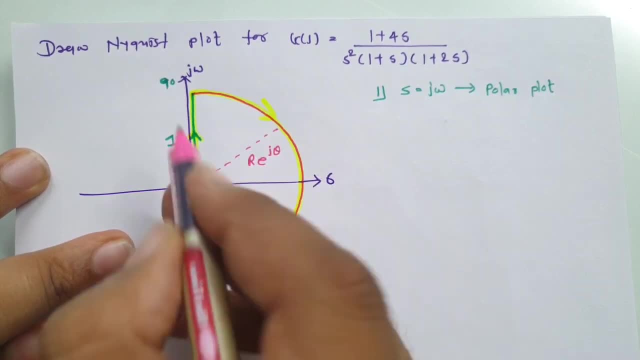 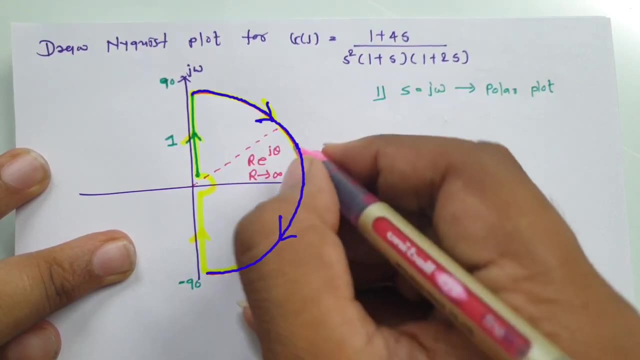 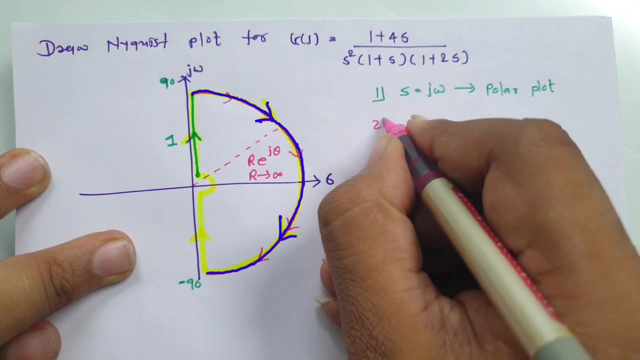 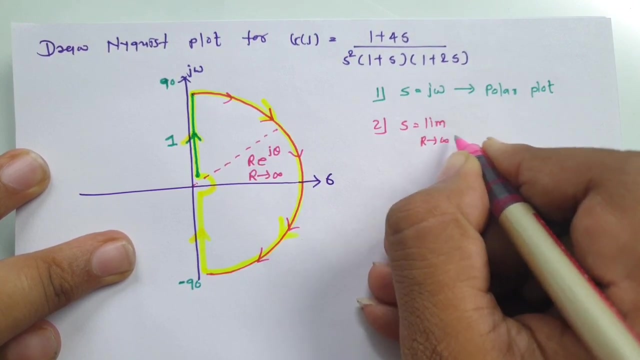 radius r and angle theta, then theta will vary from 90 to minus 90. And the radius is going towards infinite Right, So this is happening in this direction, you see, from 90 to minus 90. Right, So here we'll be placing. s is equals to limit capital, R tends to infinite, r into e, to the power, j, theta, where theta 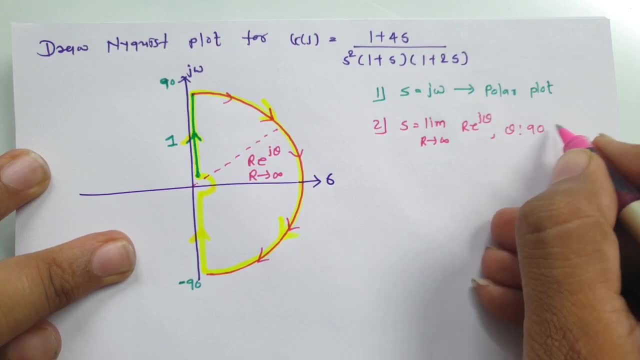 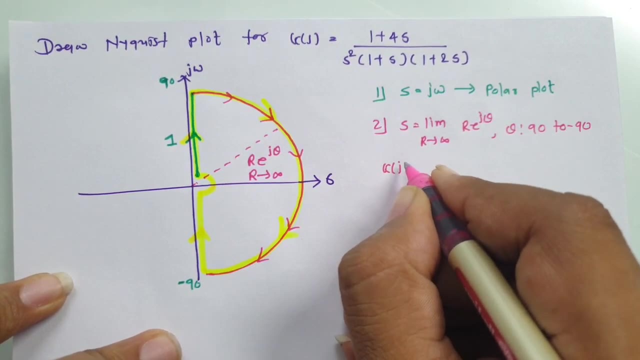 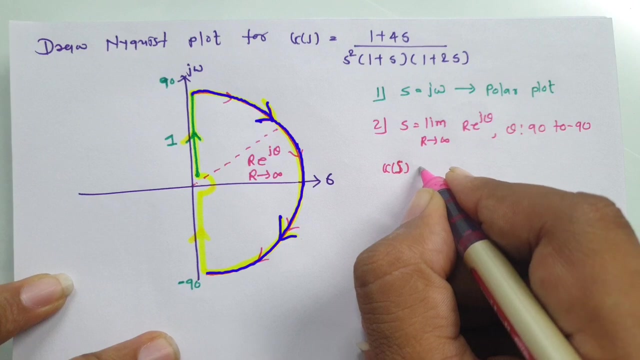 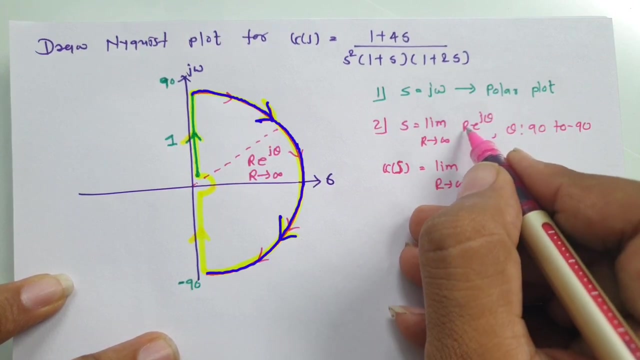 that will vary from 90 to minus 90 right, and now we will identify system. so g of s that we are to identify right, and that is limit. capital r tends to infinite. now, you see, instead of s, we will replace it by capital r e to the power j theta. so 1 plus 4 capital r e to the power j theta. 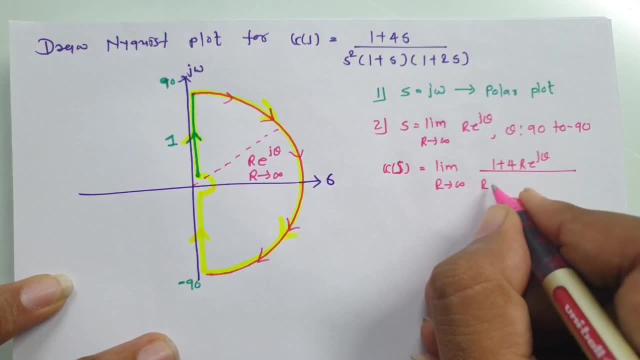 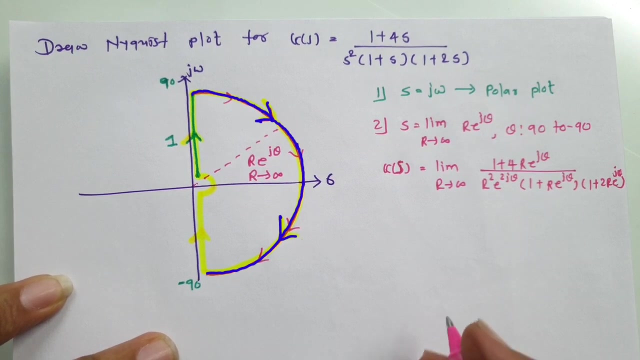 divided by s square, so that is r square e to the power 2 j theta into 1 plus capital r e to the power j theta into 1 plus 2 capital r e to the power j theta. right now, to simplify this further, what i'll be doing is: 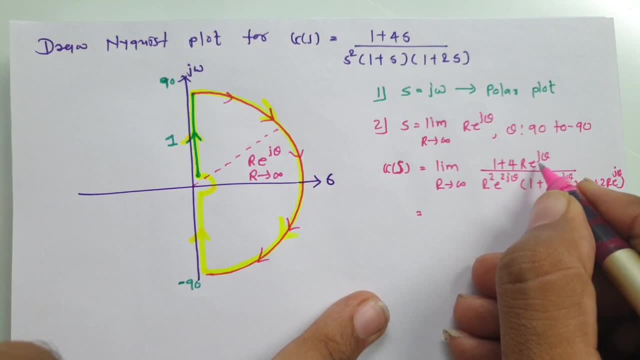 i will be play. i will be taking common r? e to the power j theta, 4 r? e to the power j theta from numerator and from here r? e to the power j theta and from here 2 r e to the power j theta, so you 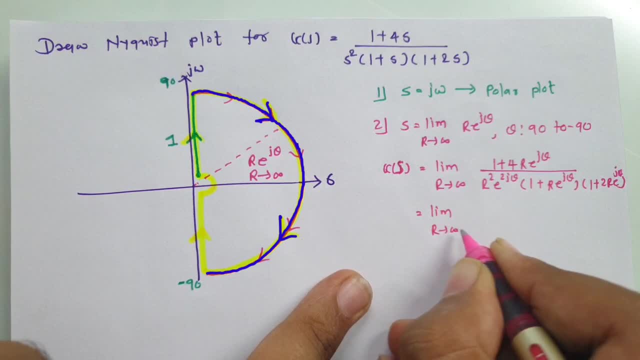 see what will happen. limit r tends to infinite. now this will become 2 divided by r cube, and e to the power j theta in numerator and e to the power j theta in numerator and e to the power j theta numerator and in denominator e to the power: 4 j theta. so in denominator it will be e to the power. 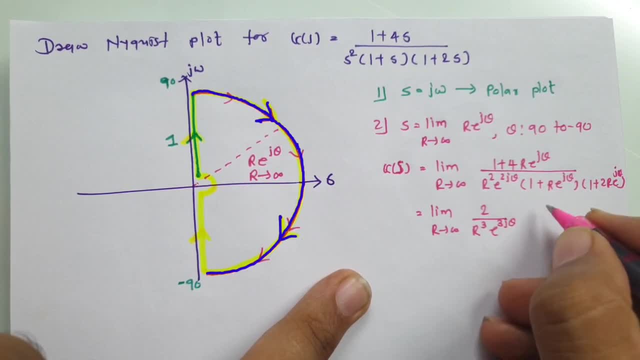 3 j theta. that will happen. and with this you see what will happen: 1 plus 1 by 4 r e to the power j theta. that will happen. and in denominator 1 plus 1 by r e to the power j theta and 1 plus. 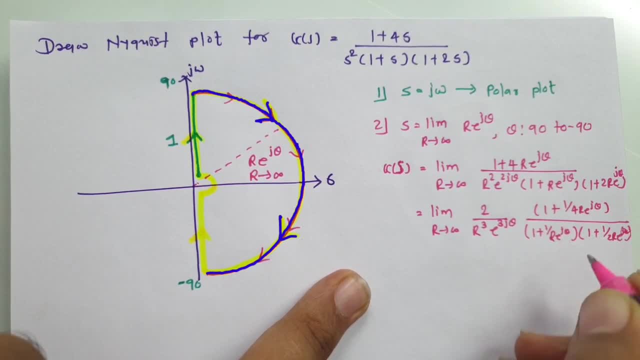 1 by 2, r, e to the power j theta that will happen and where, if you place r tending to infinity, this term will get 0. so 1 plus 0, 1 plus 0, 1 plus 0, so that will make it to 1. so simplified version of this that will be: r tending to infinite, 2. 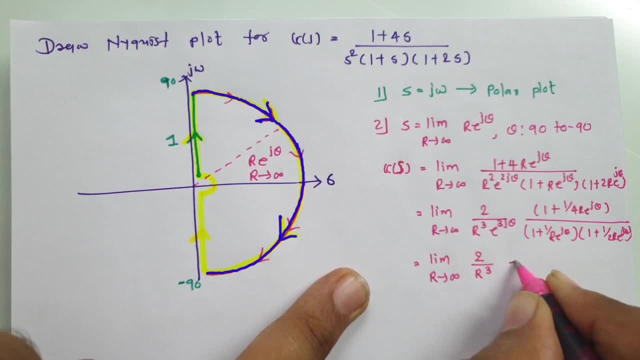 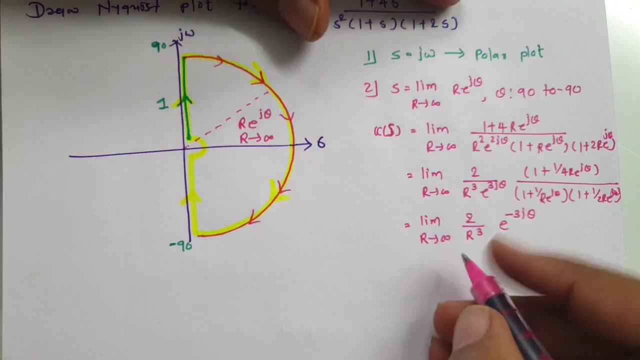 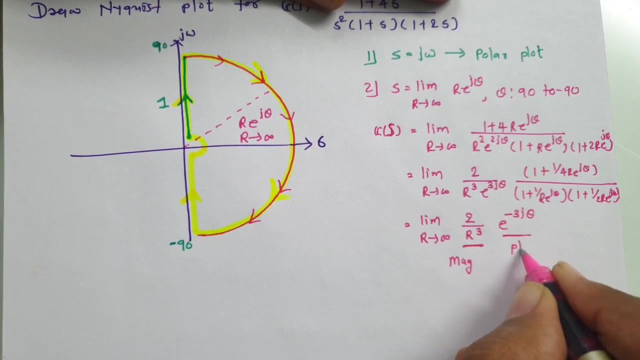 divided by r cube that is there with us, and in angle e to the power minus 3 j theta that is there with us right now. in this you see this term that explains magnitude and this term that explains phase, now, as if r tending to infinite, 1 by r cube is there. 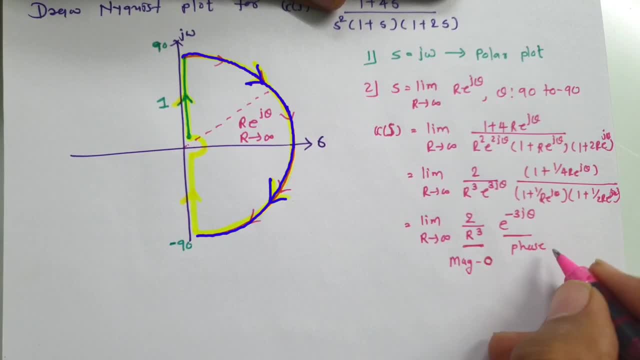 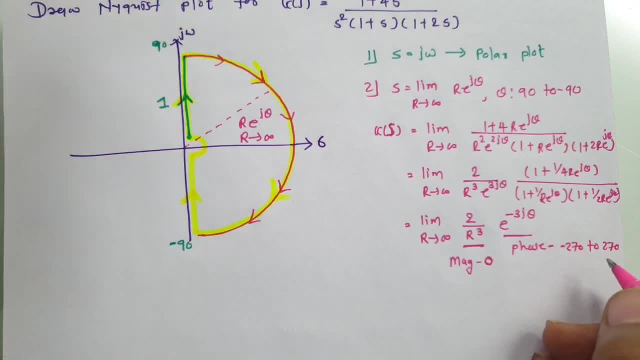 minus 90 to minus 90, to minus 90 to plus 70. so now you see, phase is changing. from minus 270 to plus 270 means here there will be 1.5 circle. 1.5 circle, and that will happen from minus angle to plus angle, means anti-clockwise direction circle. 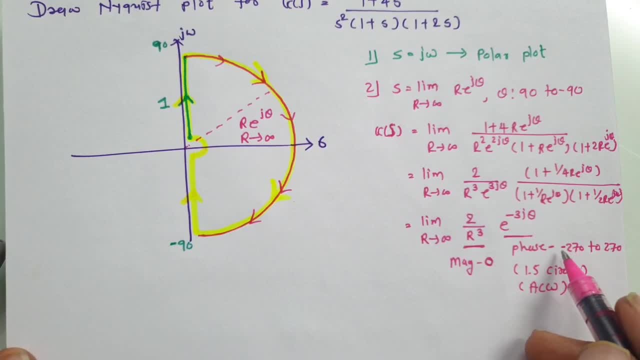 will happen. on right, if angle changes from minus theta to plus theta, anticlockwise circle will happen. and you see, minus 270 to 270 means 540 angle will change and 540 angle means 1.5 circle will happen. so in nyquist plot how to use this, i'll explain you. 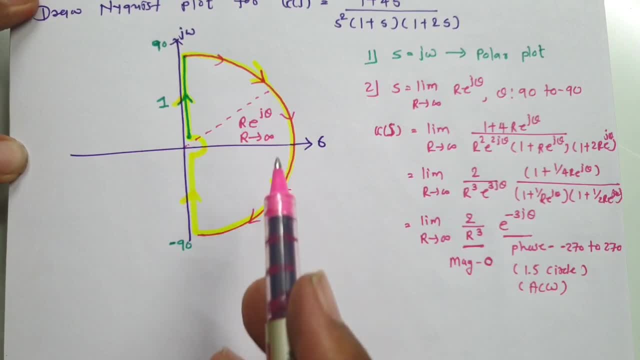 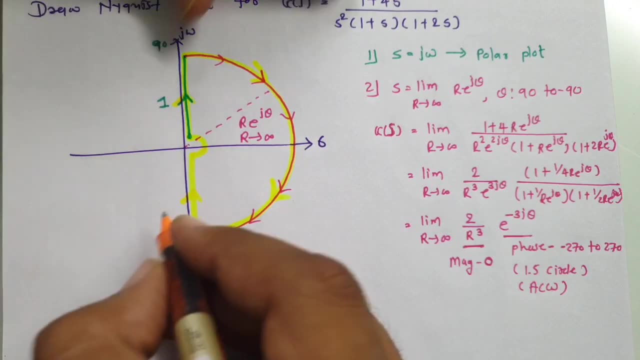 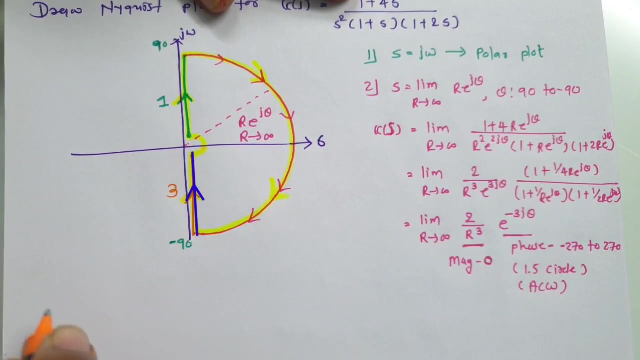 later. let us try to understand this first, and then we will apply all the steps one by one now here, if you observe this portion. so in this portion- this is third portion, and in third portion you see we are just placing- s is equals to minus j, omega, right? so what is that? 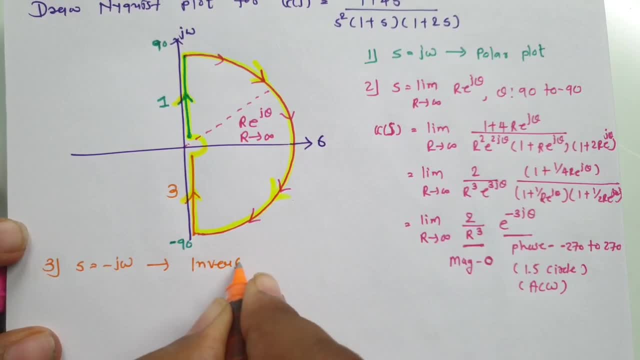 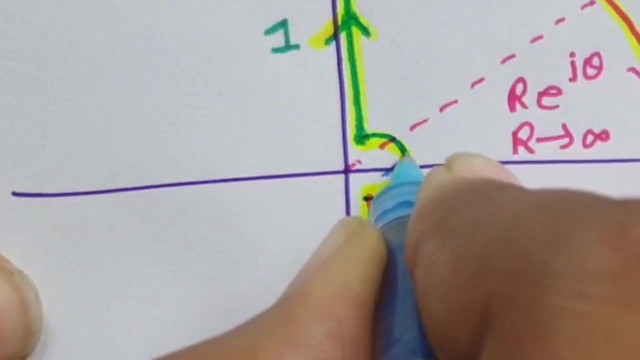 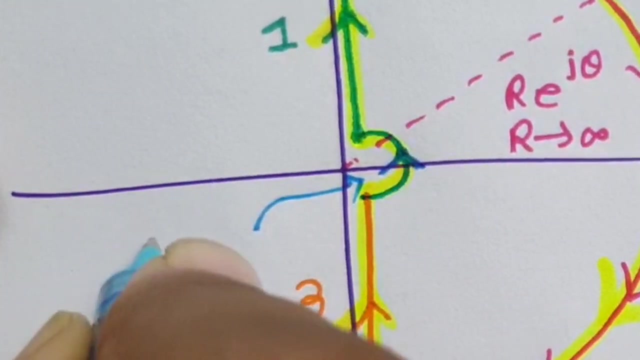 it is inverse polar plot. it is inverse polar plot, so i'll explain you how to plot inverse polar plot. so let me explain you first, fourth encirclement, that is this one. and you see that is happening in this direction, right? so if you see this circle, so this circle is having radius small r. 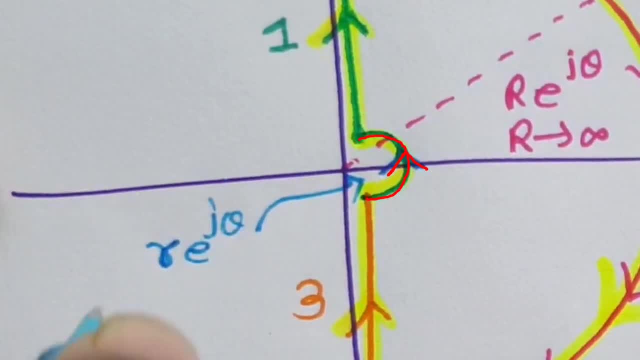 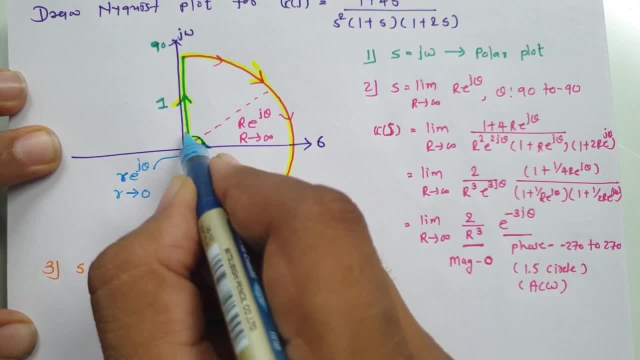 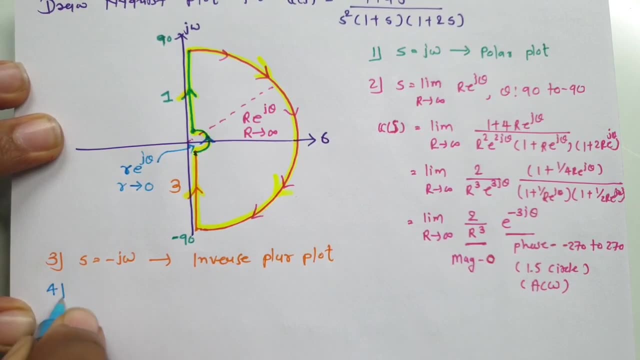 minus 90 to plus 90. you see, here angle is minus 90, here angle is plus 90, so angle varies from minus 90 to plus 90. so let me write that first. see fourth point. so in that we will have to replace: r is equals to limit. small r tends to zero. small r e to the power. j. theta, where theta belongs to. 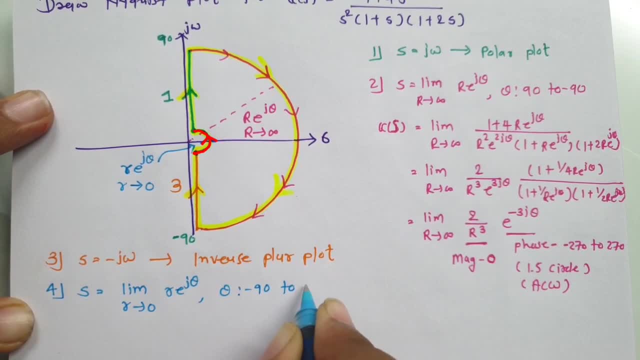 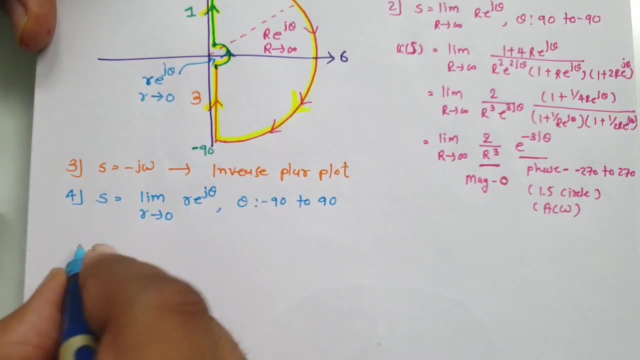 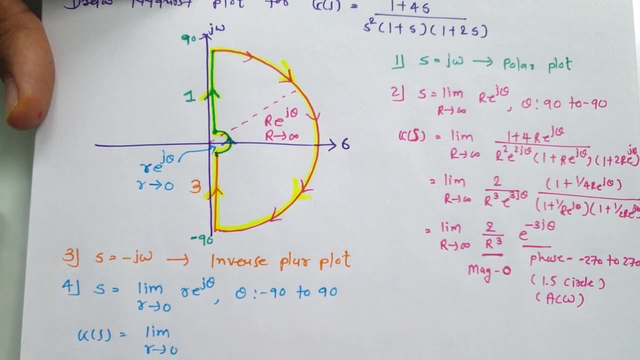 changing from minus 90 to plus 90, right, and we will have to identify system. so here now you have g of s. now that will be limit. now r tends to zero and we will have to replace s by r into e to the power j theta in this right. so let us. 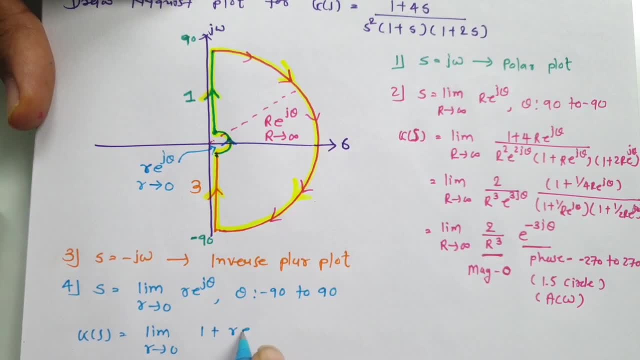 replace this one plus small r e to the power j theta divide by now s square is there. so r square e to the power 2 j theta that is there with us, and we will have to replace r into e to the power j theta into one plus small r e to the power j theta into 1 plus 2 small r e to the power j theta吧. 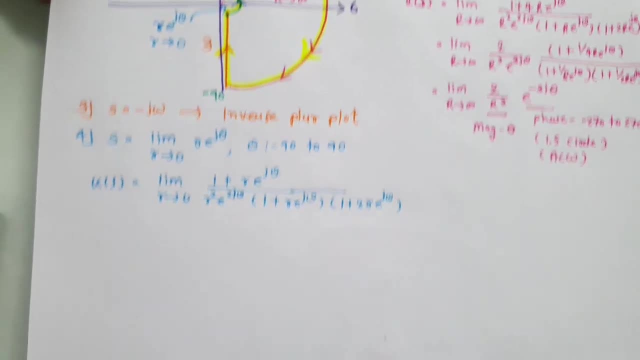 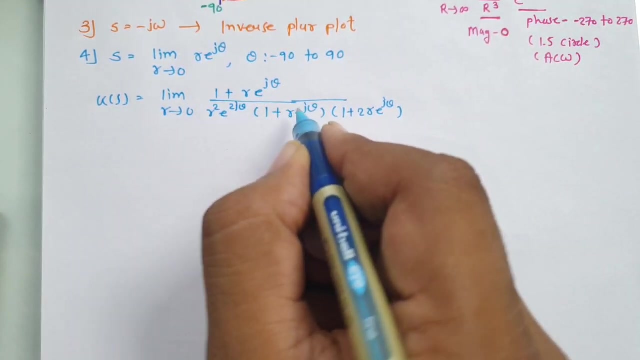 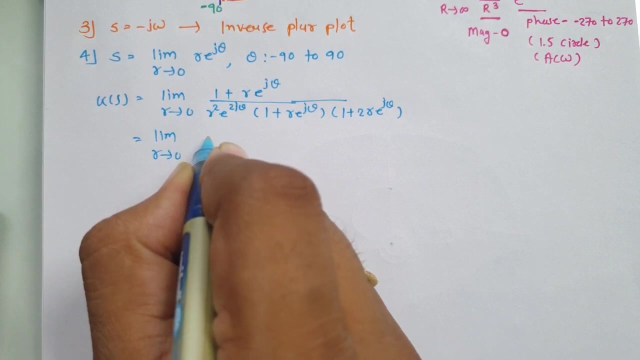 is how it is there with us right now. here you can directly provide: R tends to 0, so this will be 1 plus 0, this will be 1 plus 0 and this will be 1 plus 0, so we can say this is essentially 1 by r. 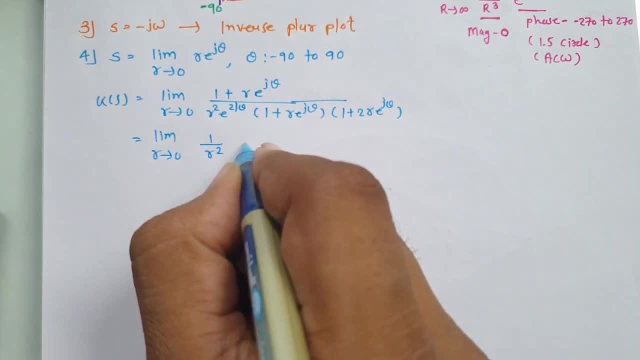 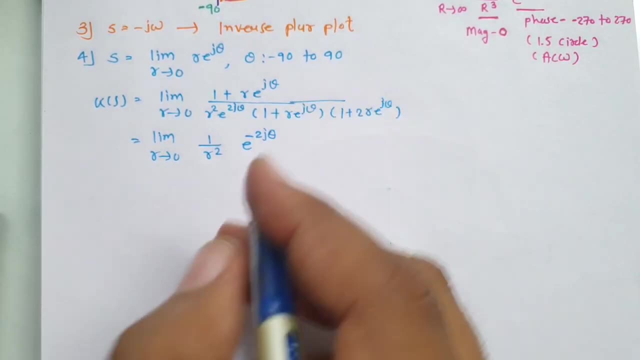 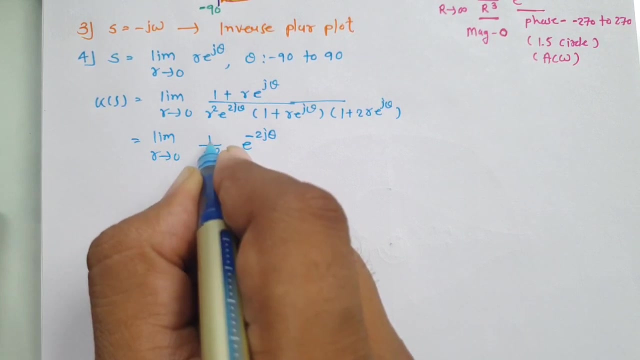 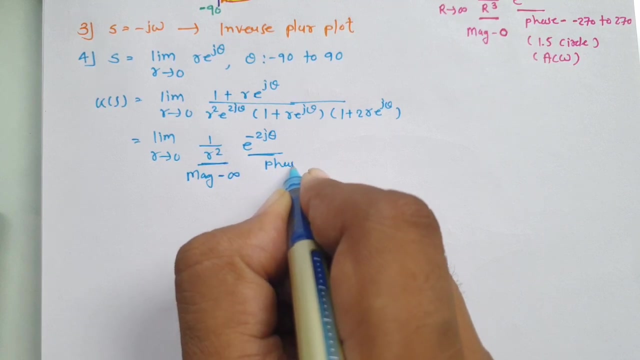 r square and 1 by e to the power of 2 j theta, so that will be over here. e to the power minus 2 j theta. right now, in this you see, this represents magnitude. and 1 by r square where r tends to 0, so that magnitude will be infinite. and this represents phase. now you see how phase 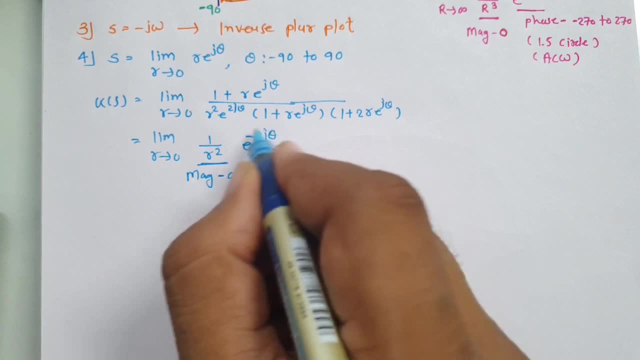 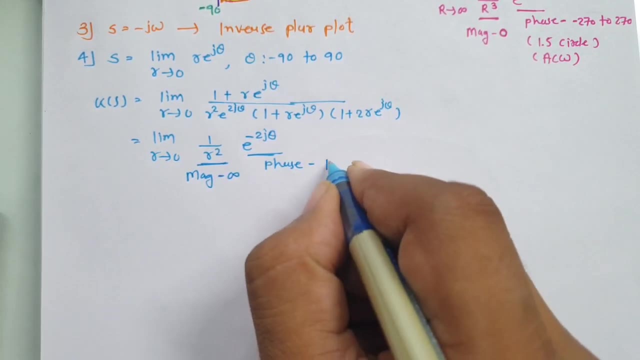 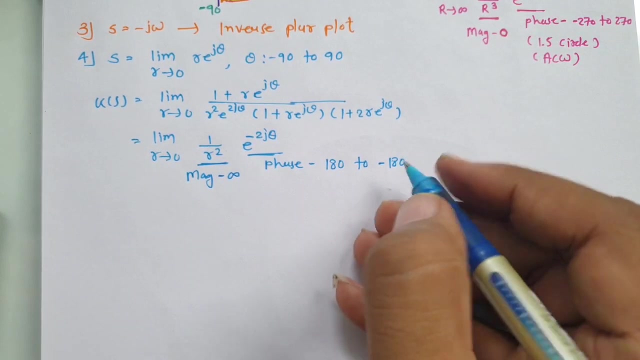 changes. so minus 2 theta. that is how phase is changing, where theta varies from minus 90 to 90, so minus 90 into minus 2, so that is 180 to 90 into minus 2, so that is minus 180, so 180 to minus 180. 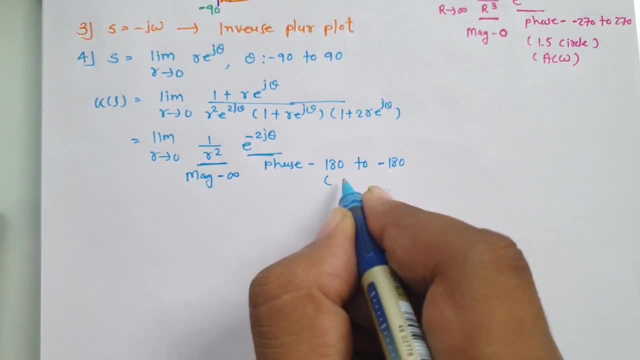 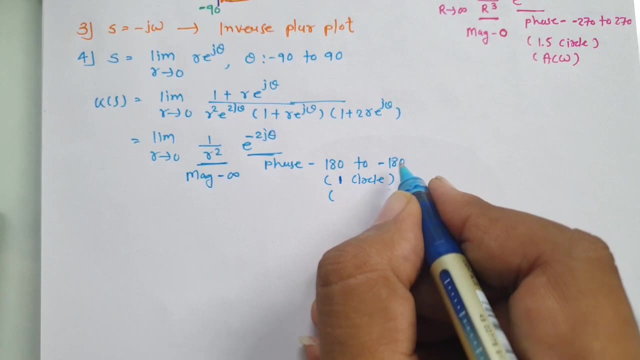 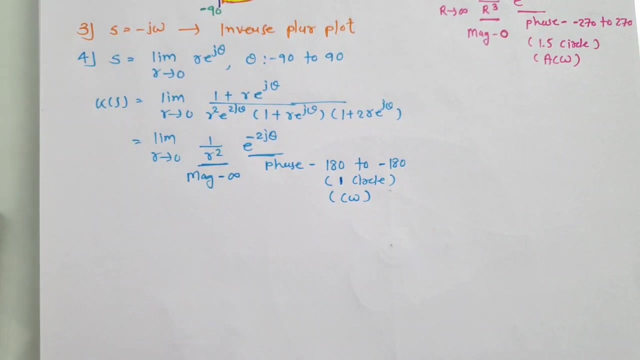 angle will change. means total 360 degree angle will change, means one circle will happen. and you see, plus 2, minus angle variation is happening. means clock over 90 degree angle will change. so that is how phase changes. so minus 2 theta, that is how clockwise circle will happen. clockwise circle will happen right now, as i have said. see there. 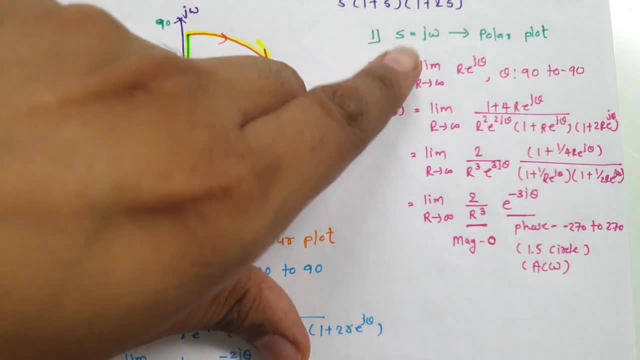 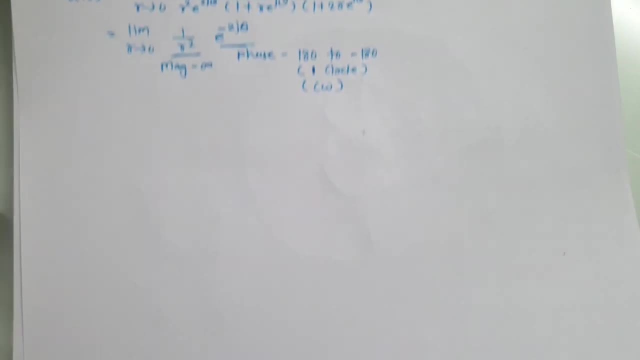 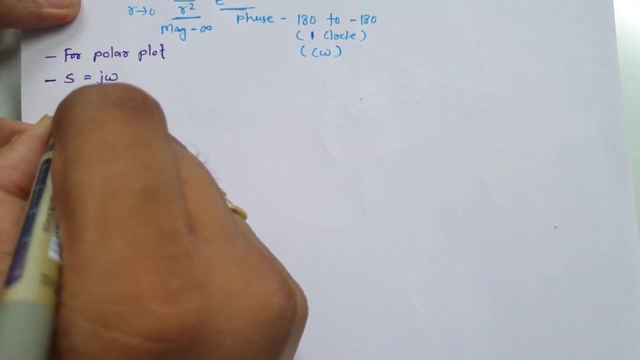 are four steps that we need to follow and one step, that is to have polar plot, which we need to identify now. so now, once we identify polar plot, we can have nyquist plot for this question, right, so, let us have polar plot. so now we have g of j, omega. that will be 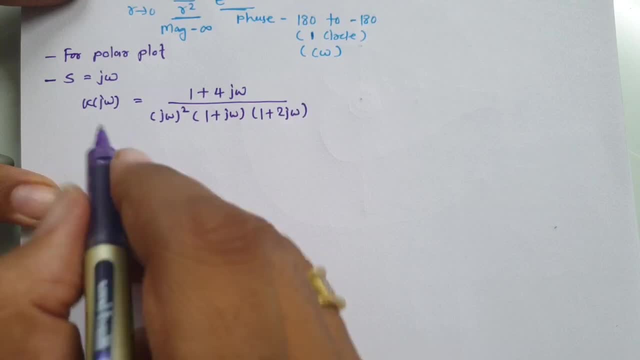 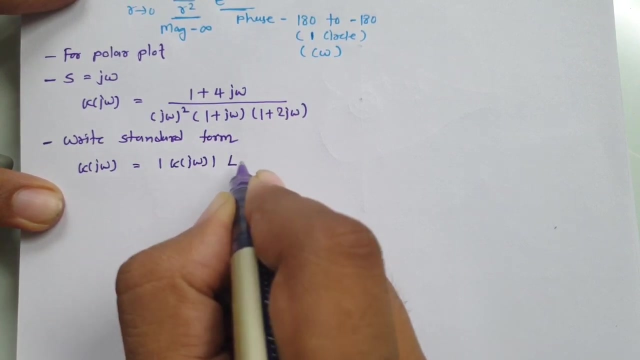 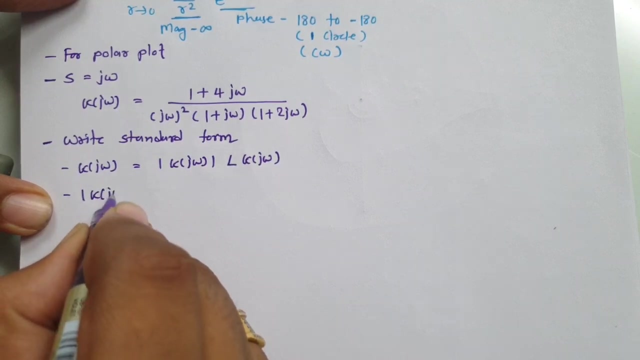 so this is g of j omega that we have. now second step, that is, to identify standard form of this equation. so standard form that is magnitude of g of j omega into phase of g of j omega. now here, if you observe magnitude of g of j omega, so that will be square root of for. 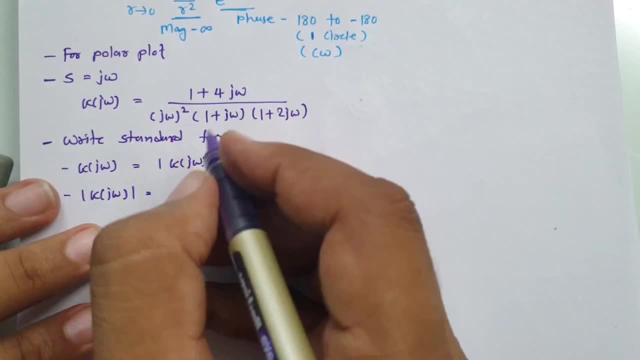 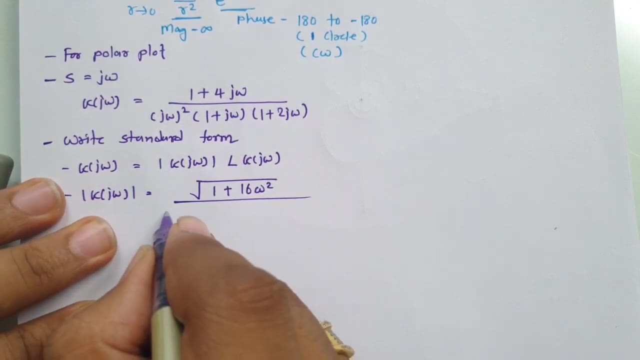 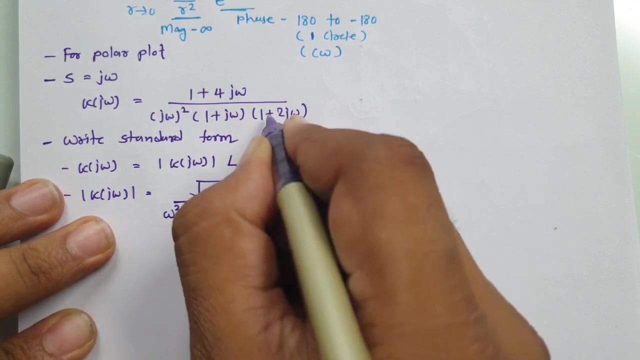 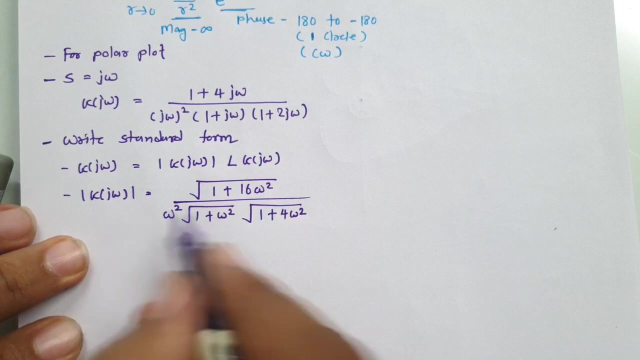 magnitude and now we need to identify phase. so you see we have square root of 1 plus j omega square. so niveau, it will be real component square plus imaginary component square. so 1 plus 16 Omega squared. So divided by, you see, j Omega square. 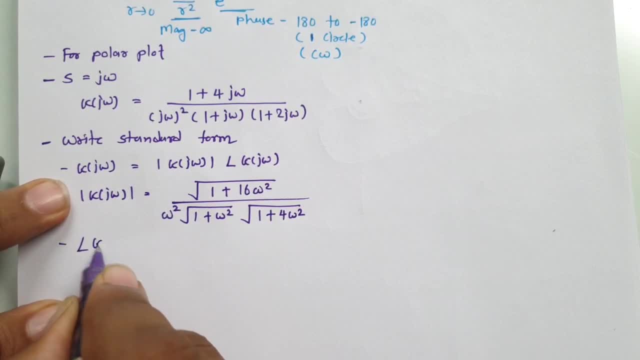 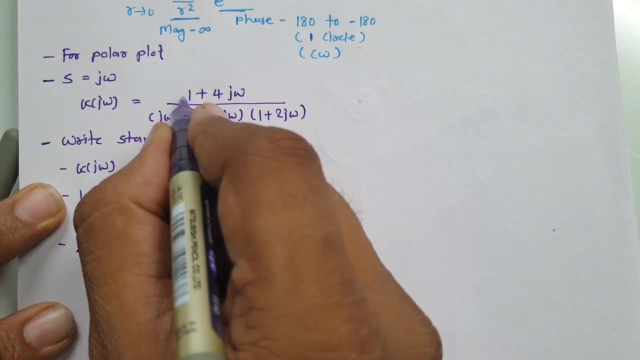 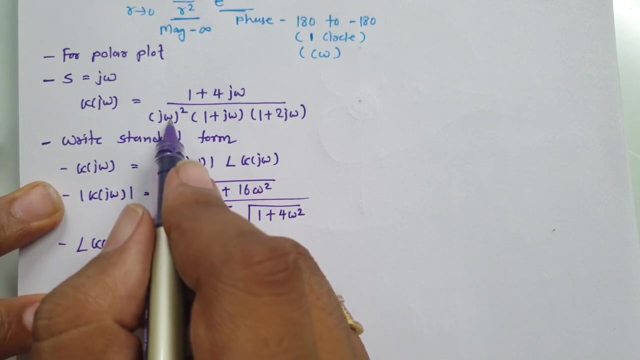 d5 phase. so you see, phase will be g of j omega. now for numerator we have zeros, so phase will be positive. so plus tan inverse, 4 j omega, so 4 omega divided by real, that is 1. right now. you see, at zero location there are two poles, so pole is having minus angle for one. 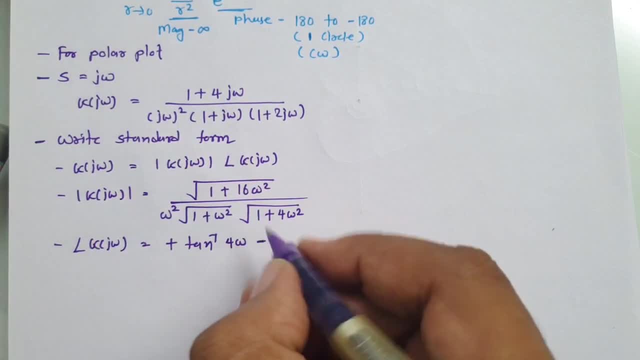 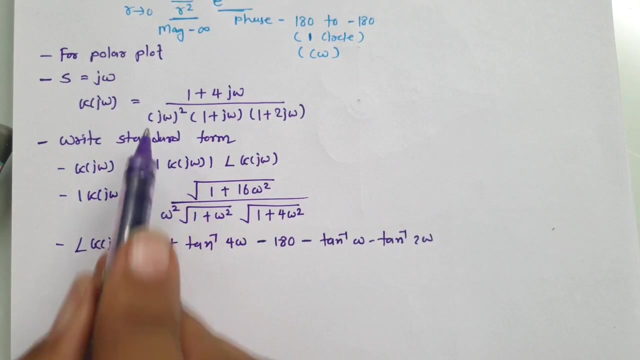 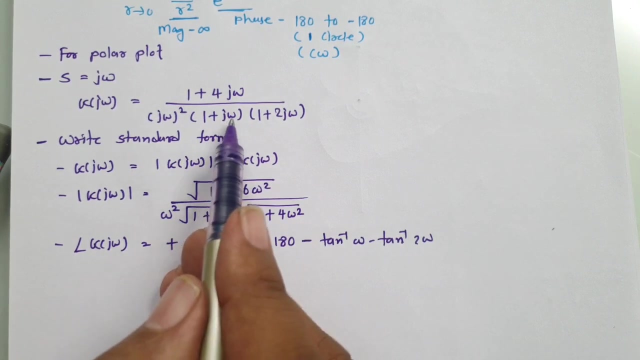 two poles at origin, there will be minus 180 degree angle, minus tan inverse omega, minus tan inverse 2 j omega, right. so if you have one pole at origin, 90 degree, if you have two pole at origin, minus 180 degree, angle will be there and tan inverse imaginary by real, so tan inverse 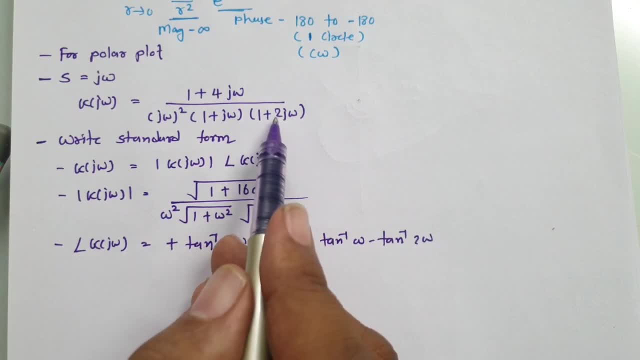 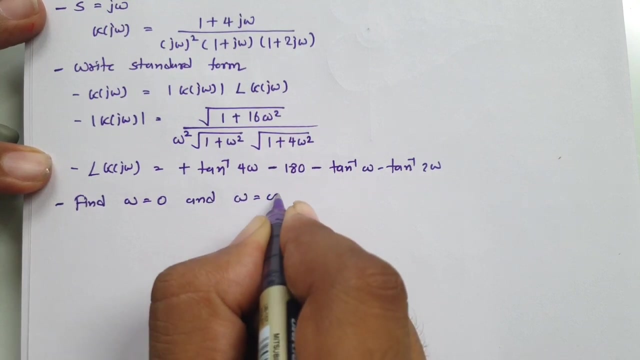 omega. tan inverse imaginary by real. so tan inverse 2 omega by 1. so that is tan inverse 2 omega. right, so that is how phase is there with us now. in next step we will have to identify two essential points, and those two essential points are there at: omega is equals to 0 and 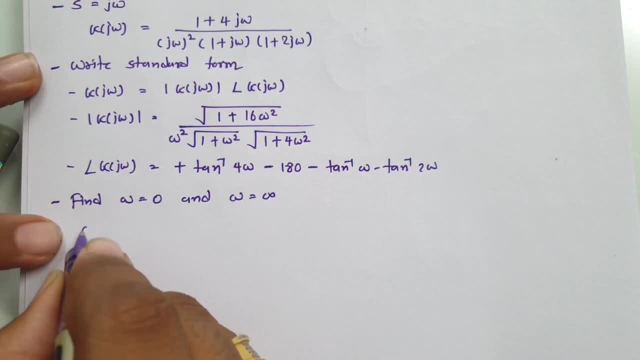 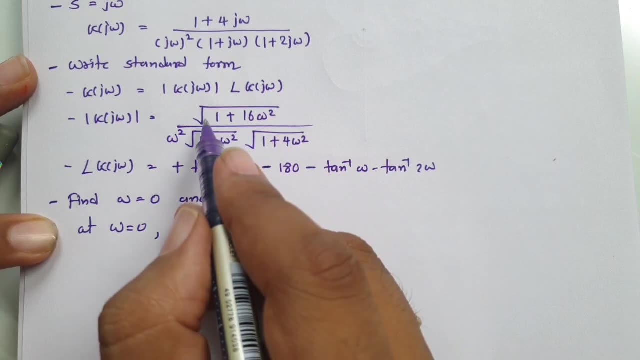 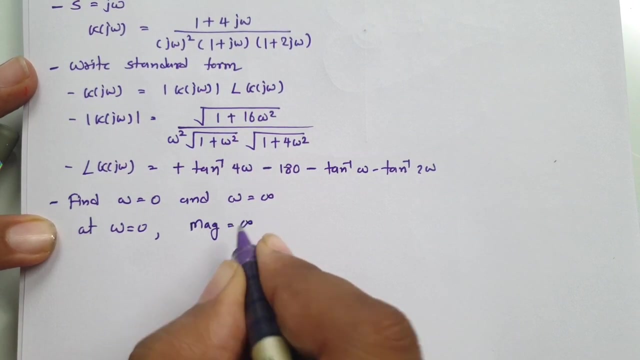 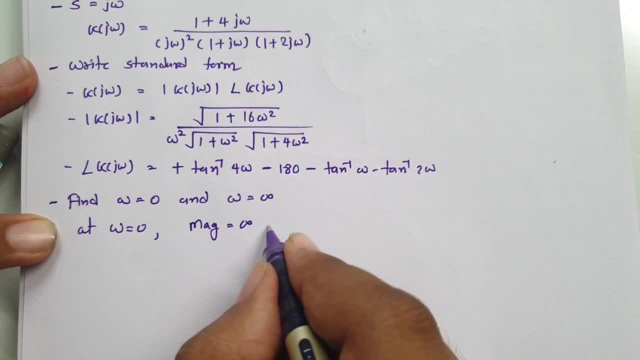 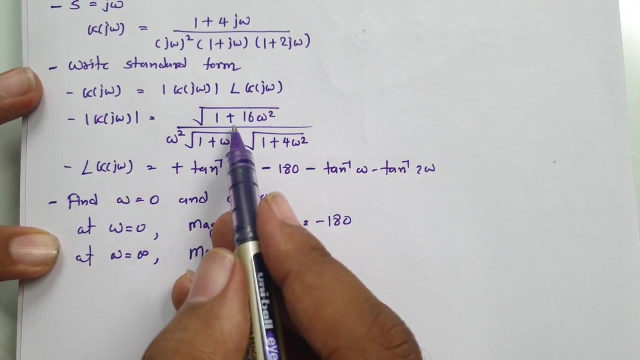 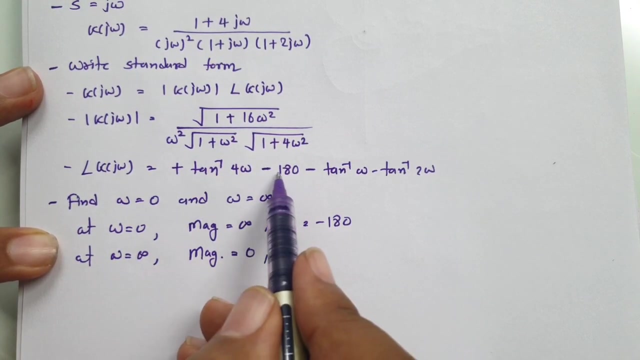 see 0 minus 180, minus 0 minus 0, so phase will be minus 180 at this point. and second essential point that is happening at omega is equals to ifinite. so where what is magnitude? so you see, if you take that 1 by in finite as denominator having higher order, we can say: magnitude i will be 0 and phase that will be 90-180-90-90. so that is minus 270 degree. 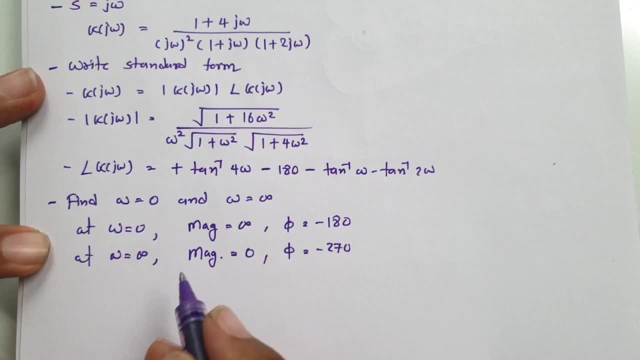 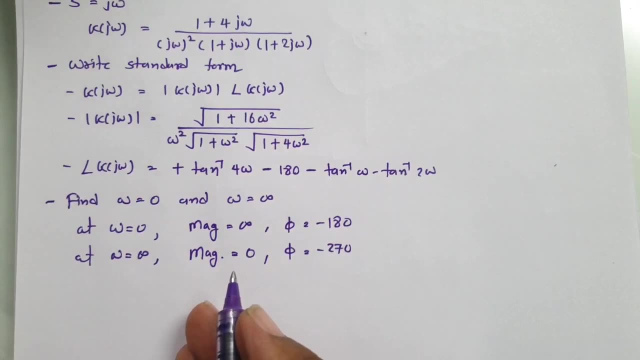 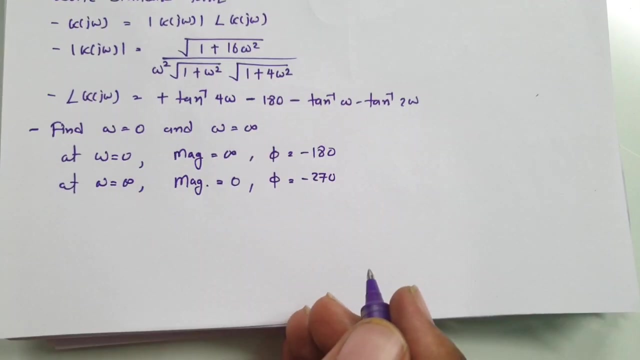 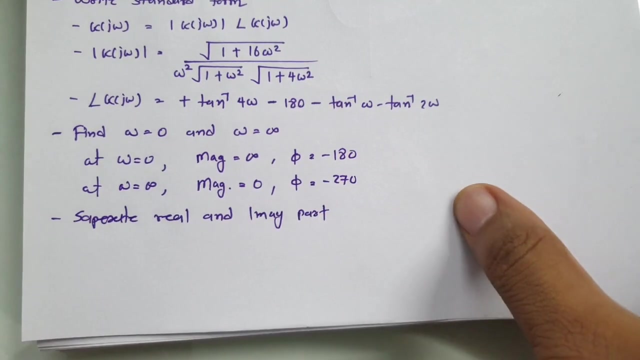 right. so now we have two essential points now to identify intersection to real and imaginary axis. all we need is we need to have separation of real part and imaginary part, right? so in next step we will separate real and imaginary part. so now I'll explain you how to separate. 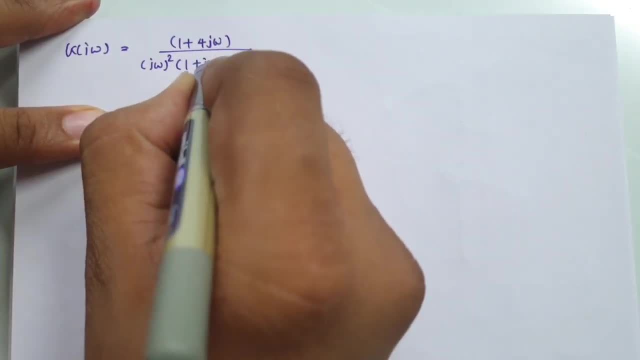 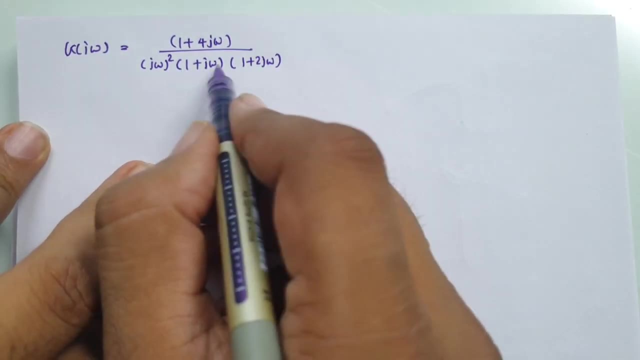 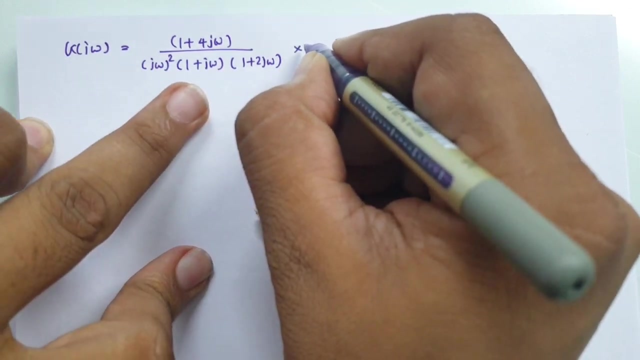 real and imaginary part. now see to separate real and imaginary part. all we need to do is for denominator. we need to multiply and divide complex conjugate of denominator, right? so here you see: 1 plus j omega. that is there in denominator, so I'll be writing 1 minus. 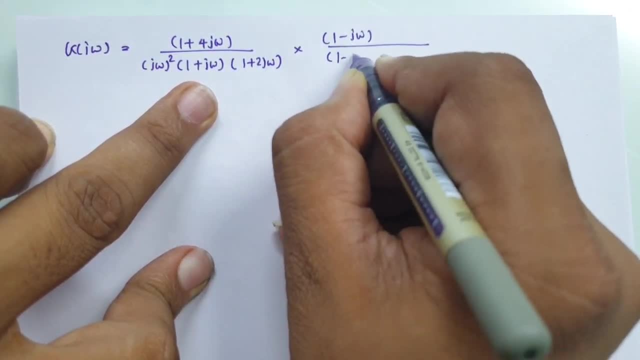 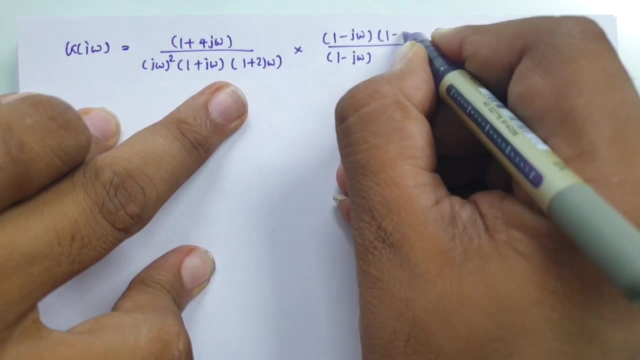 j omega and I'll be dividing 1 minus j omega. and you see, in denominator 1 plus 2 j omega is there. So I'll be multiplying 1 minus 2 j omega and I'll be dividing 1 minus 2 j omega. so what? 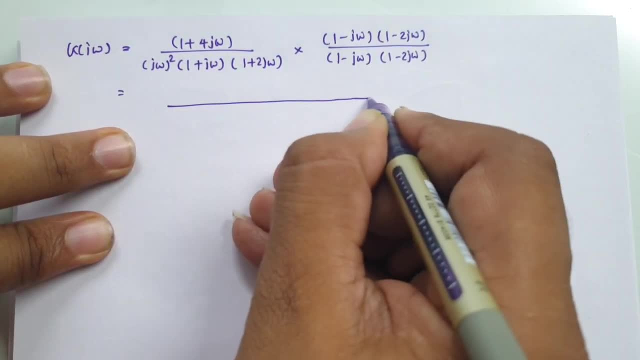 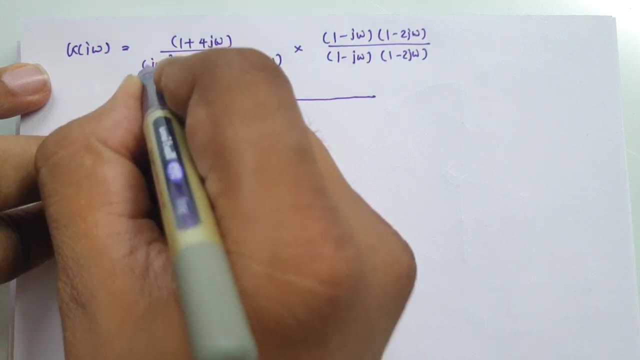 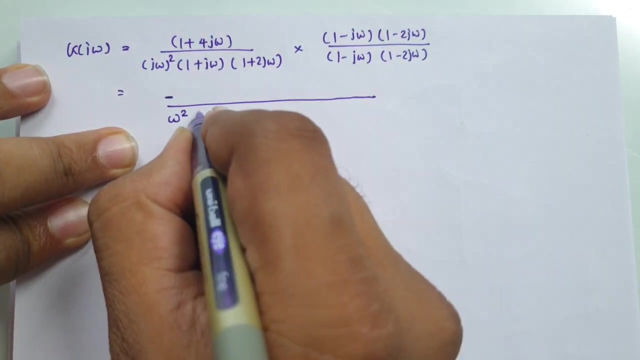 will happen. you see, now in denominator. now in denominator, see, this is j omega square. so we can say it is omega square and j square is minus 1. so I'm writing minus over here and 1 plus j omega into 1 minus j omega. that is 1 plus omega square. right, it will be 1 minus. 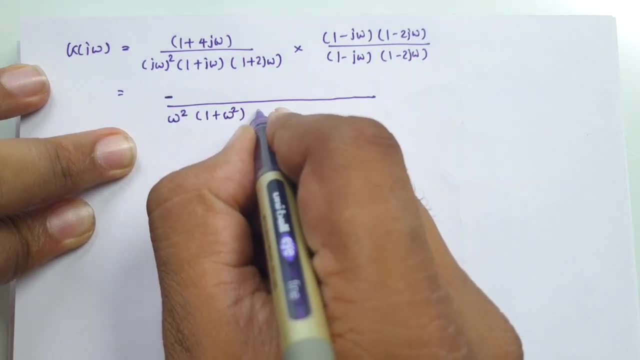 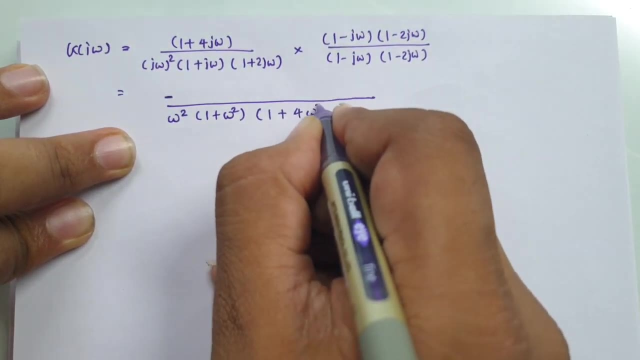 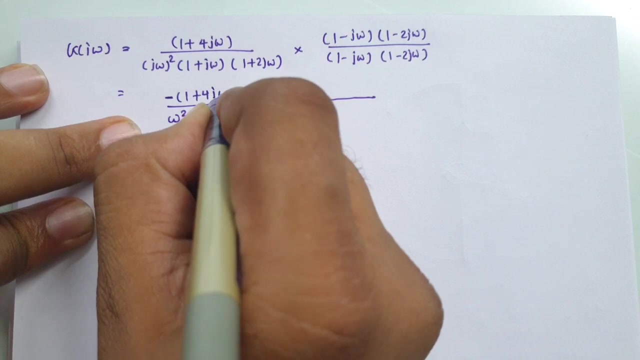 j square. omega square, j square is minus 1. that's why and you see 1 plus 2 j omega into 1 minus 2 j omega, so that will be 1 plus 4 omega square. Now first I'll write this: 1 plus 4 j omega and let us separate this term. so you see this: 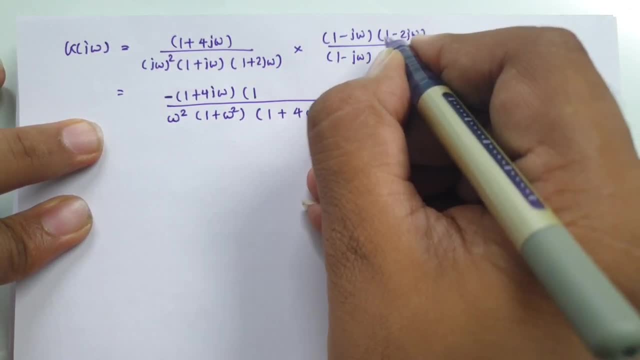 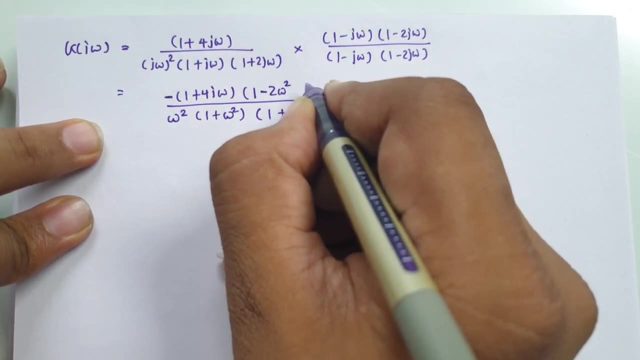 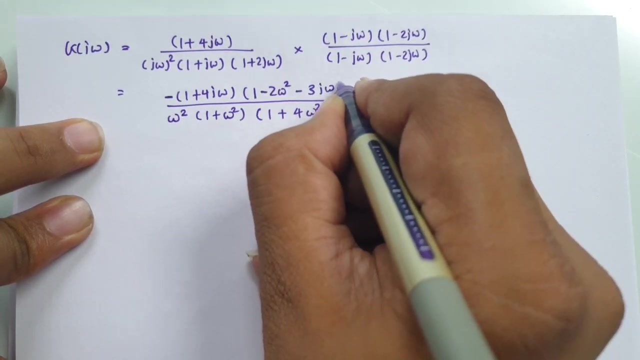 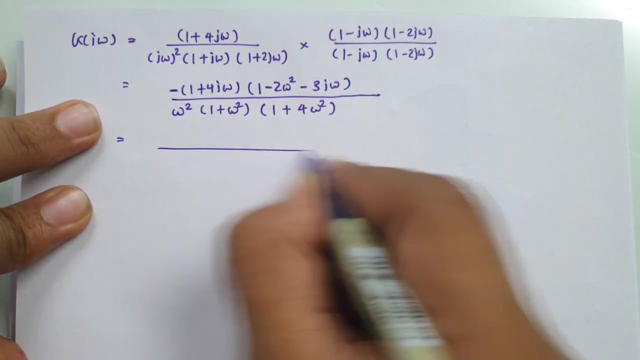 will be 1 minus minus plus j square is minus 1.. So minus 2 j 2 omega square and minus j omega. minus 2 j omega, so that will be minus 3 j omega. right now, let us separate. this counts also, so you see, this will be minus 1. let us multiply. 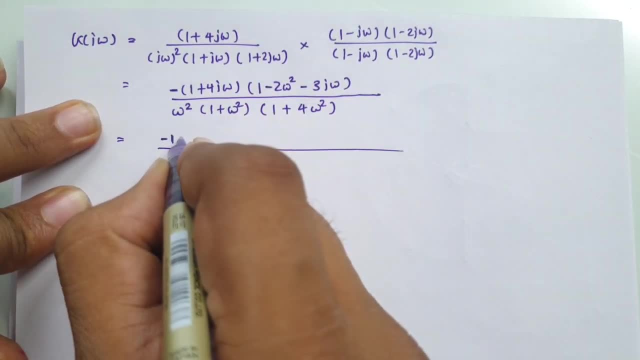 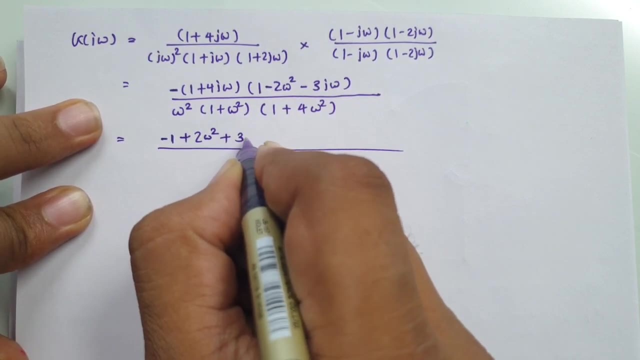 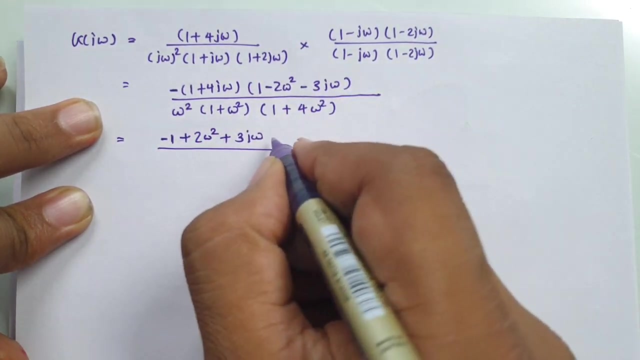 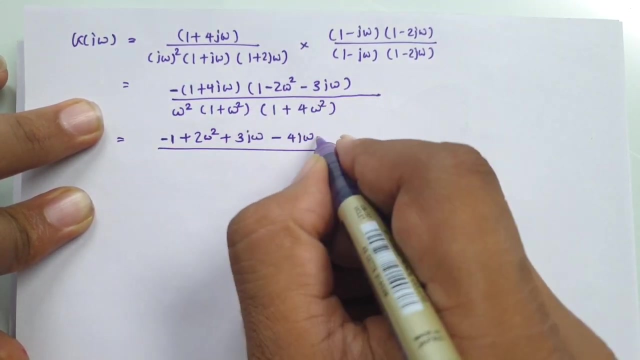 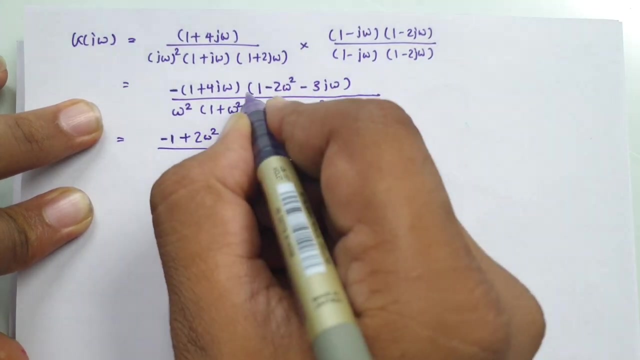 this 1 with this along with minus sign, so minus 1 plus 2 omega square plus 3 j omega. right now let us multiply minus 4 j omega with this, so minus 4 j omega, minus minus plus 8 j omega cube, and 4 into 3, so that is 1 minus 4 j omega square. 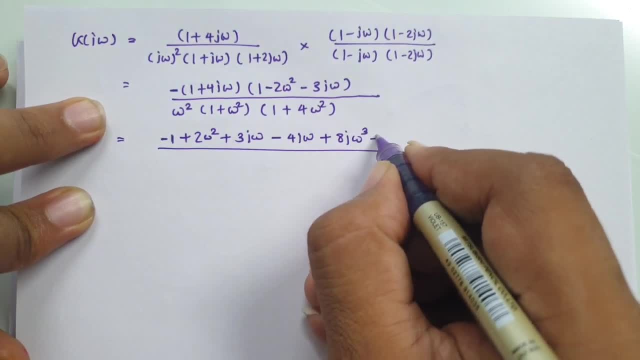 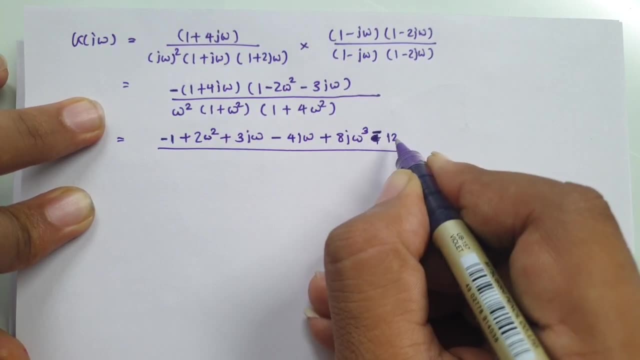 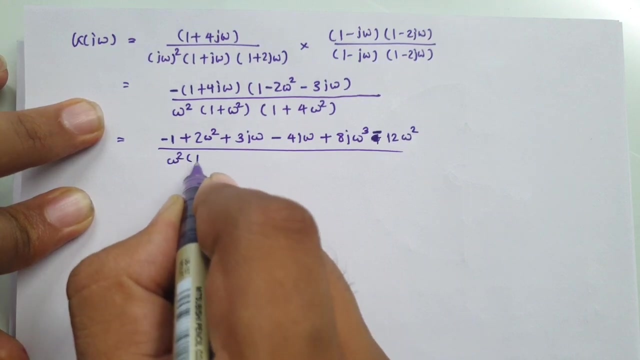 So this will be 1 minus 2 j omega square. So this will be 1 minus 2 j omega square plus 12 j square. so j square is minus 1. so minus that I'm writing now and omega into omega. so that is omega square divided by omega square. 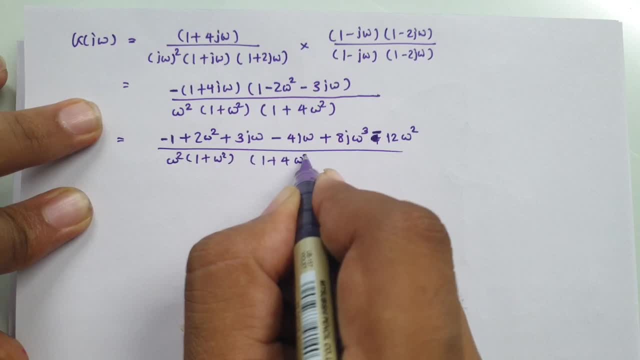 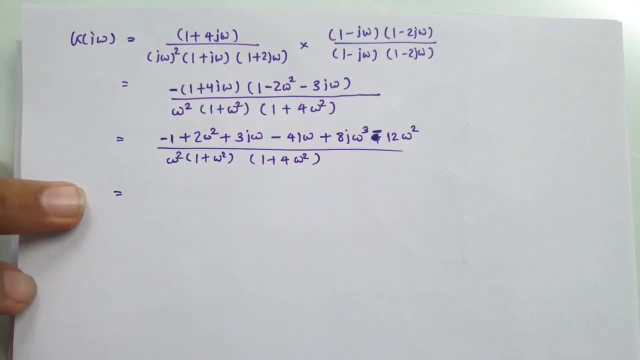 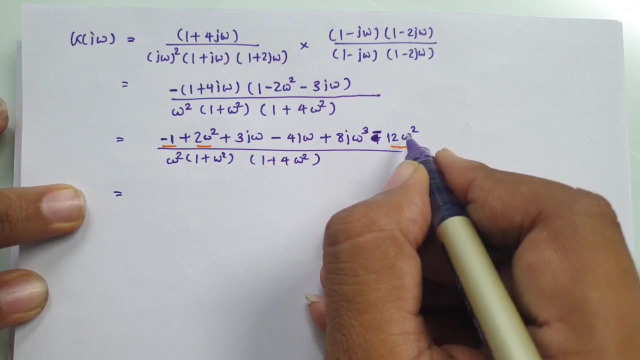 into 1 plus omega square, into 1 plus 4 omega square. right Now, take real and imaginary part separately. So now you see, for real part We have this, This and this, so in that we can say this is minus 12 omega square plus 2 omega square. 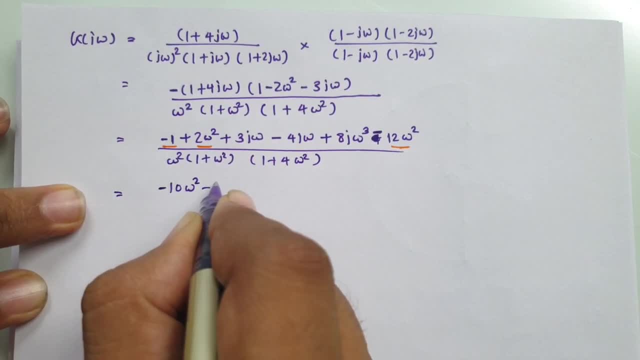 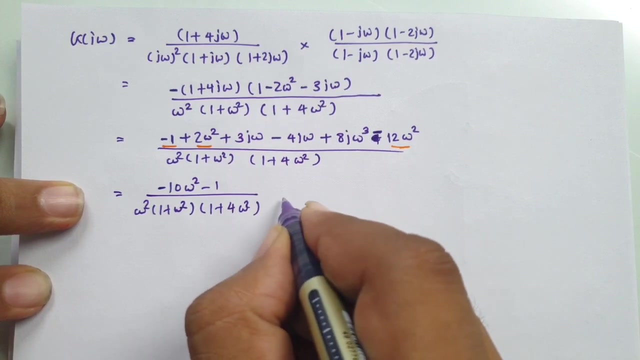 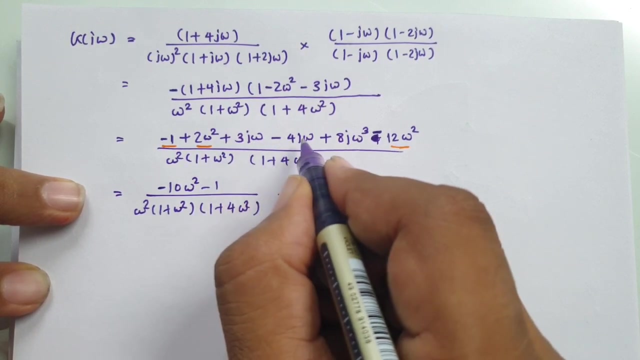 so that is minus 10 omega square minus 1 and this divided by omega square into 1 plus omega square into 1 plus 4 omega square and imaginary part. that is this. So I'm just writing plus j over here and you see this is 3 j omega minus 4 j omega, so that 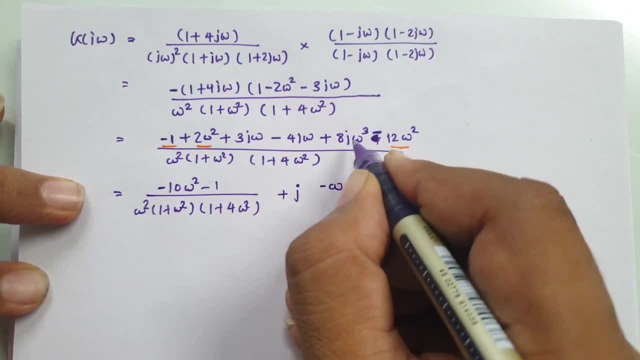 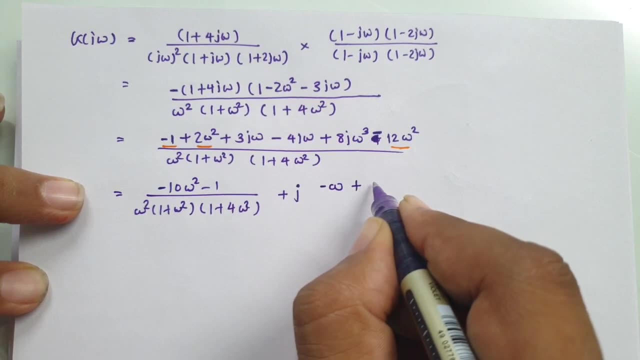 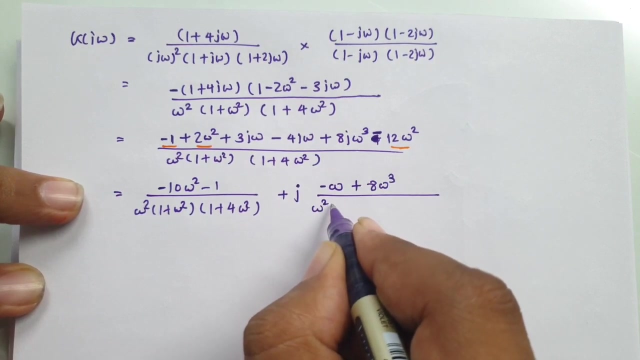 is minus omega and you see this is 8 j omega cube. So I can say plus 8 omega cube and this divided by this entire term, so that is omega square into 1 plus omega square. Now you see, from this term, 1 omega that will get cancelled over here. 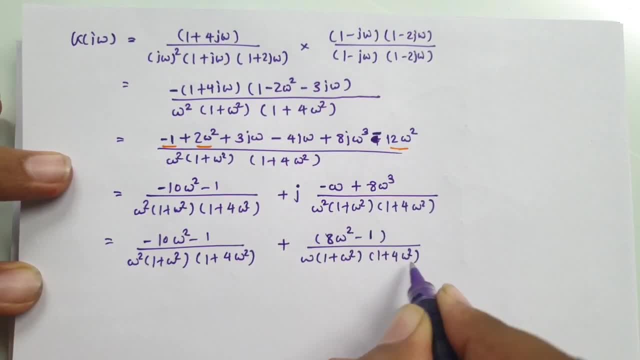 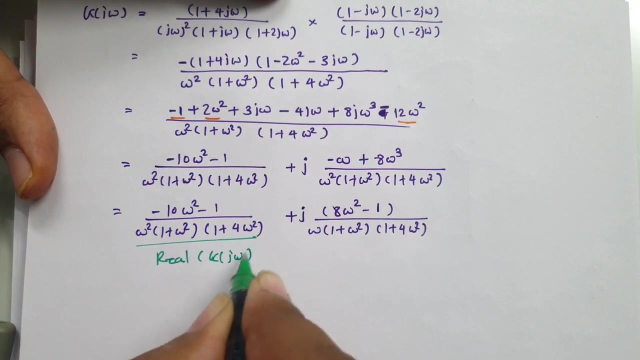 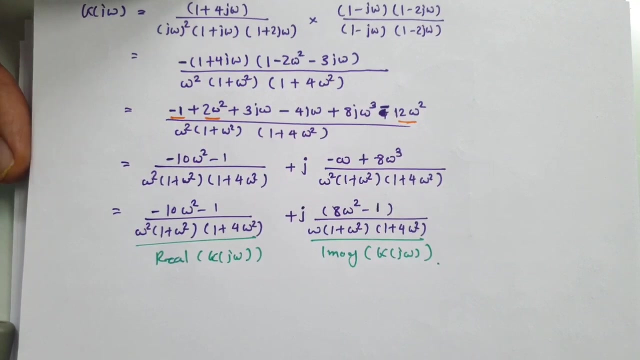 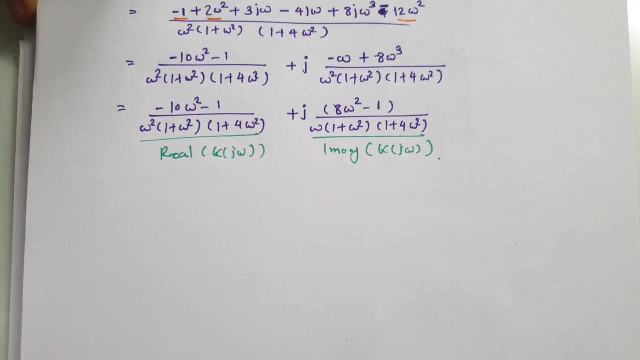 So let me rewrite that. So now you can see 1 omega that we have cancelled from numerator and denominator and this is imaginary component. So now one should know this is real component and this is imaginary component of j, of j omega. Now you see, based on real and imaginary component, we can easily identify intersection to real. 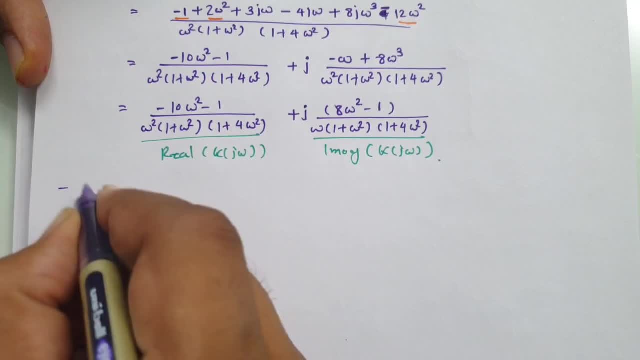 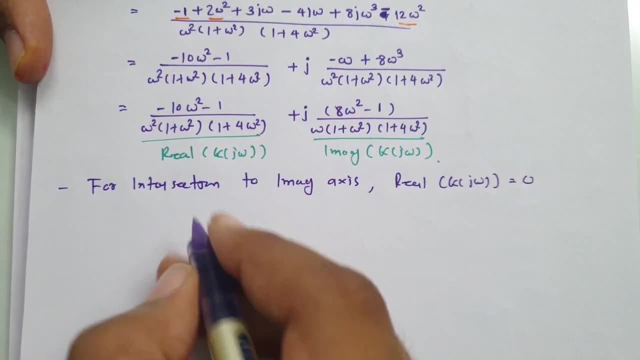 axis and intersection to imaginary axis. So in next step, to have intersection to imaginary axis, real component should be 0. So if you equate this to 0 minus 10, omega square is equals to 1. so we have: omega is equals to plus or minus j. 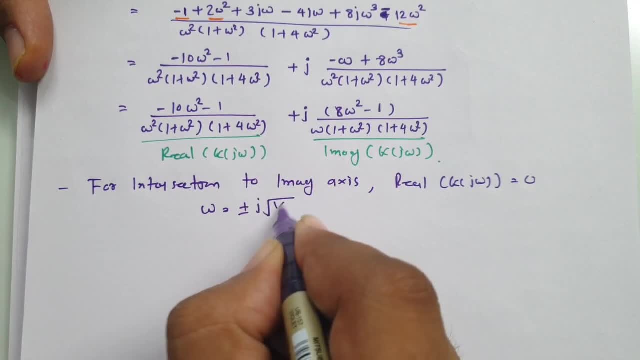 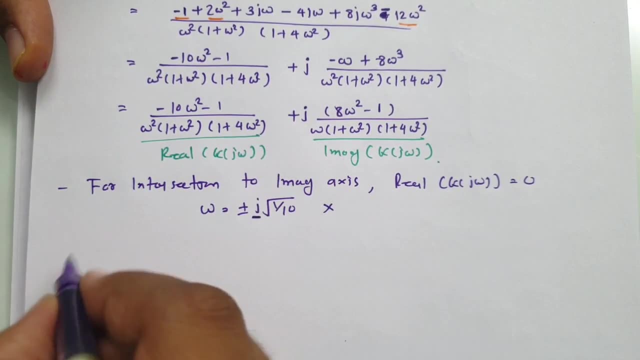 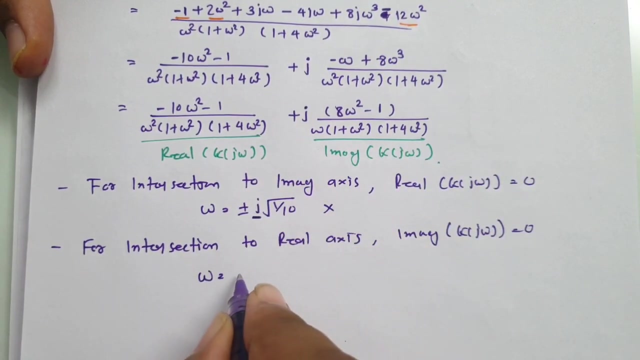 Okay, Square root of 1 by 10. but you see, frequency cannot be imaginary, right? So this is not possible. and for intersection to real axis, imaginary component should be equals to 0.. So if you equate this to 0, we have omega is equals to. you see, it will be 1 by square root. 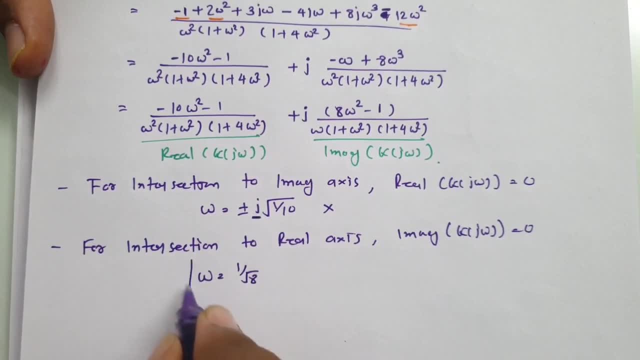 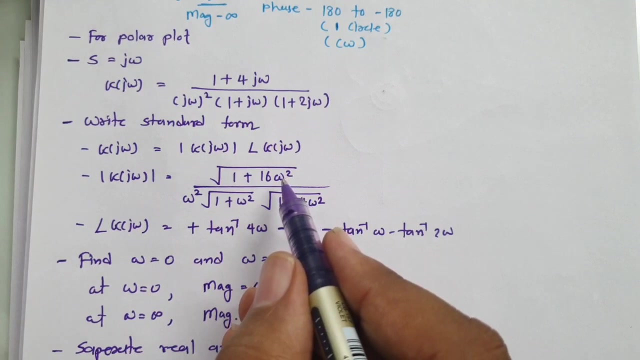 of 8, right. So now, this is what our intersection, Now, at this intersection, all we need is we need to identify magnitude and phase. So if you place omega is equals to 1 by root 8, you will be having magnitude in this. 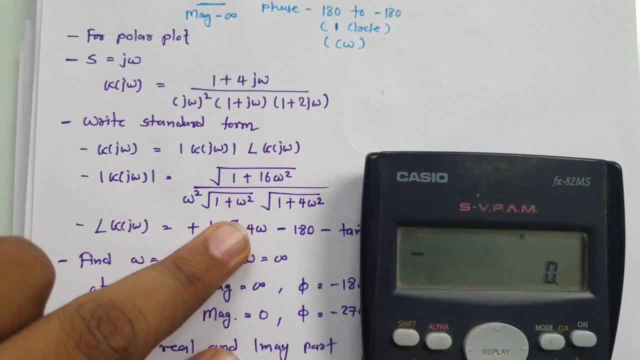 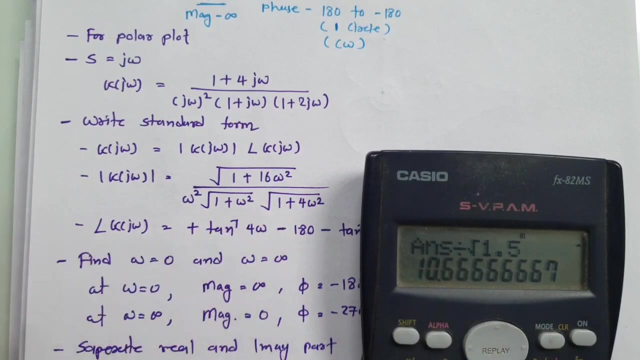 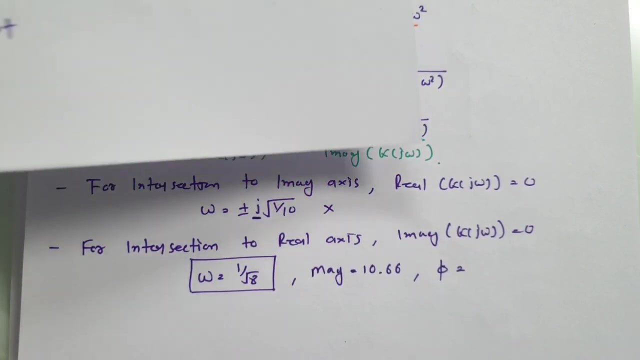 So let me calculate that in calculator, where I will be placing omega is equals to 1 by root 8.. So that is 10.66, right? So this is 10.66.. So let us place that magnitude and let us find phase. 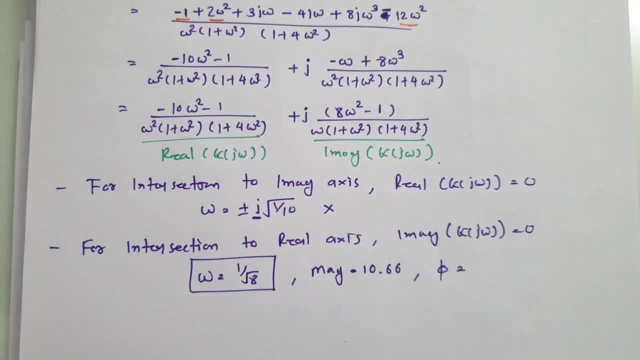 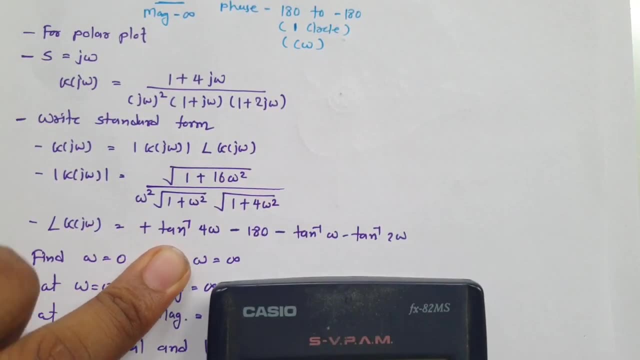 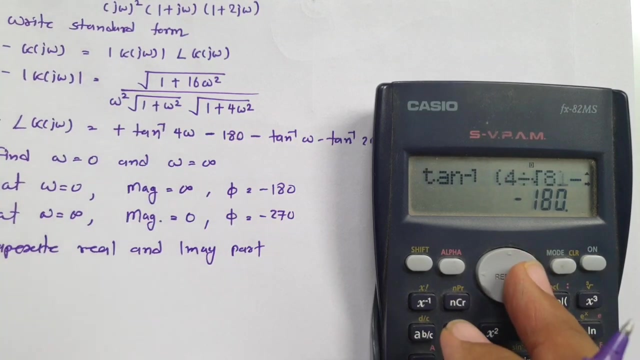 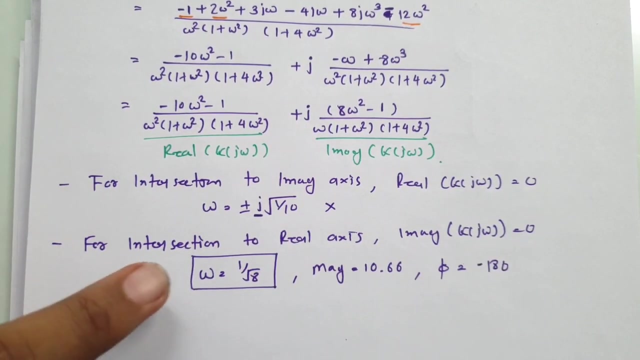 So 1 by root 8 that we are delivered to place it in phase. So here we have a phase equation in this will place that this is having angle minus 180.. I have placed it, You can see. so phi is having minus 180 angle at intersection to real axis, right. 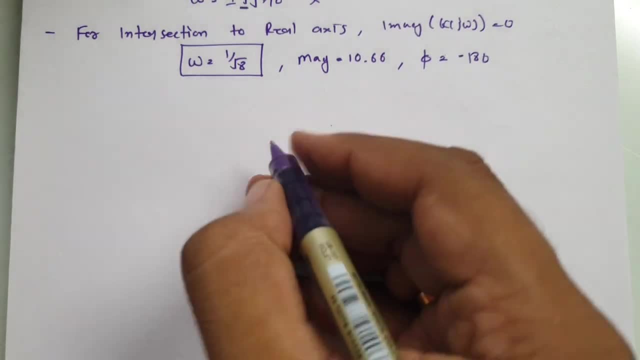 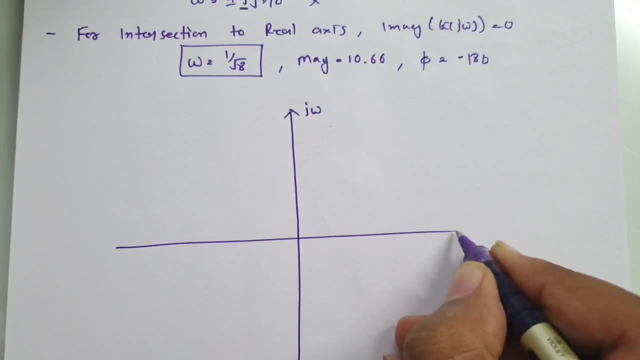 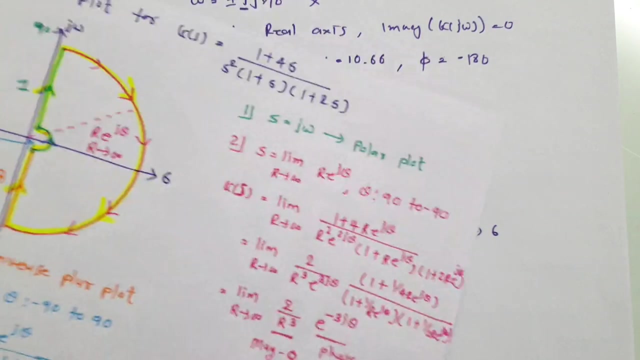 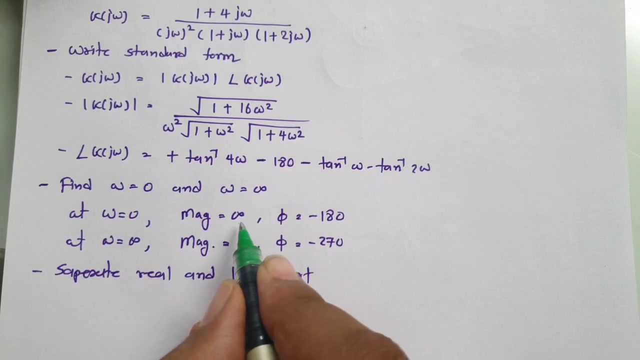 Now I will explain you how to plot Nyquist plot, step by step. So you see, here we have imaginary axis and here we have real axis. Now see, first is polar plot. So if you have polar plot First, is polar plot right. So in polar plot at, omega is equals to 0, magnitude is infinite and angle is minus 180. 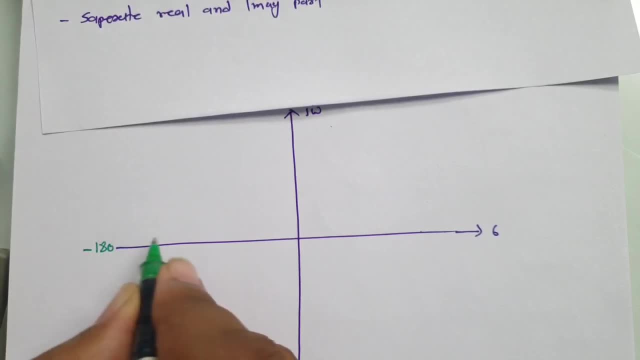 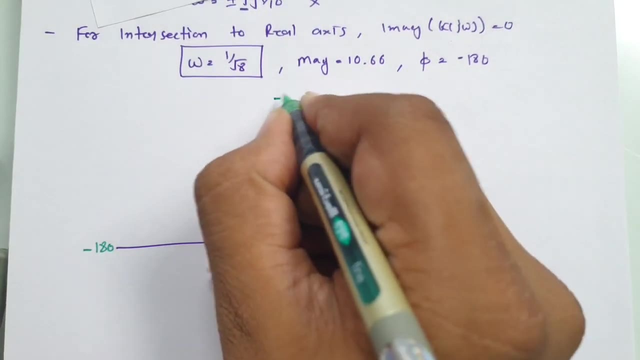 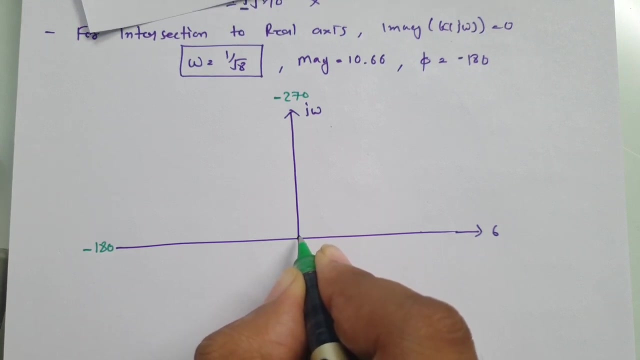 So minus 180 is happening somewhere over here. magnitude is infinite and at omega is equals to infinite. magnitude is 0 and angle is happening from minus 270. minus 270 is happening here, So magnitude is 0.. So it will be coming at 0 over here, right at minus 270. 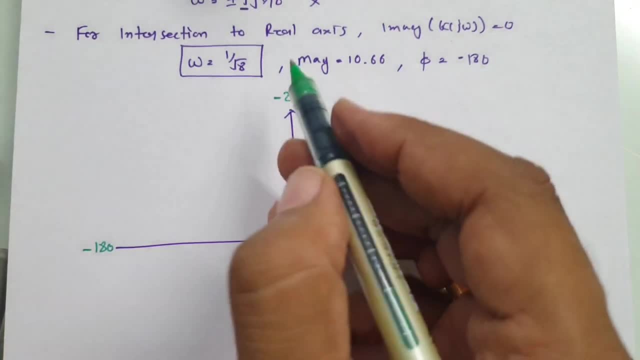 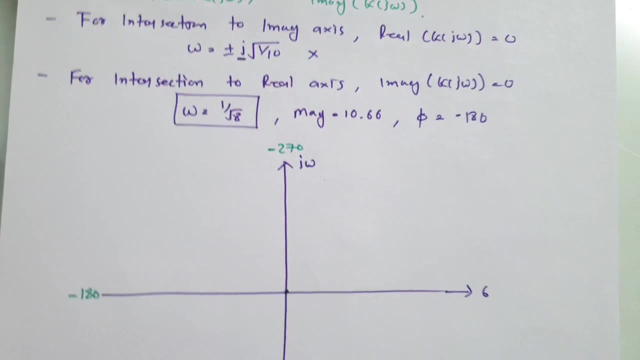 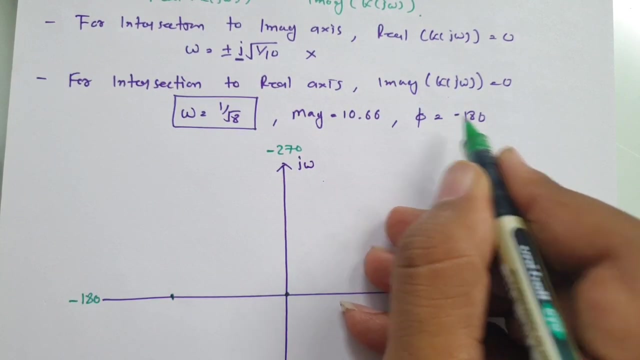 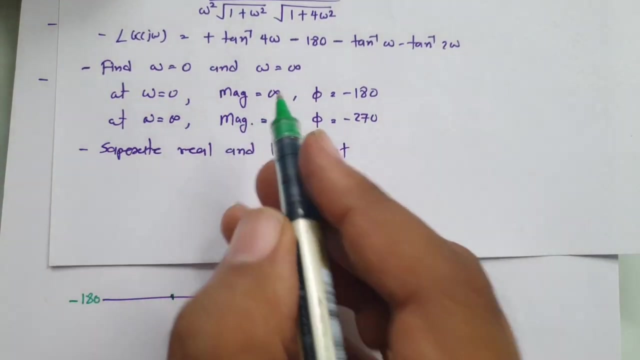 Angle. and here you see intersection to imaginary. that is not happening, but intersection to real is happening. So intersection to real, that will happen somewhere over here, with magnitude 10.66 and angle minus 180, right? So you see it will start from omega is equals to 0, magnitude infinite. from somewhere over. 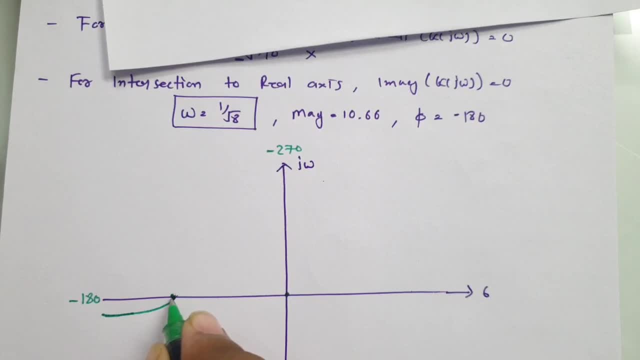 here, Right? So it will start over here and it will come here, right, And this is what a point. which is minus 10.66.. So this is our polar plot, where here omega is equals to 0, is there with us and here omega. 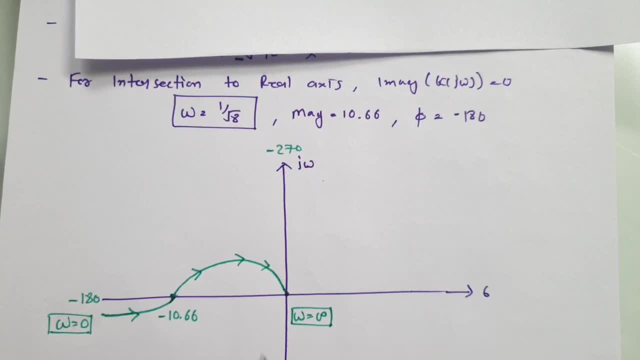 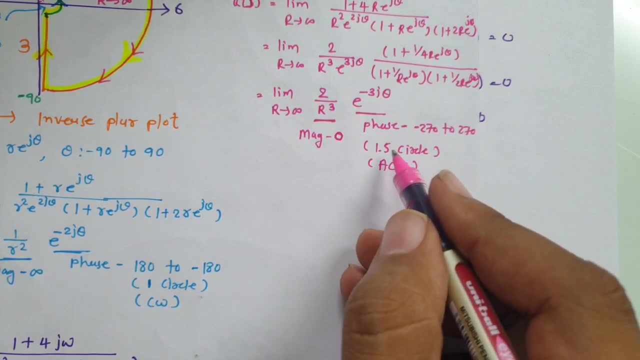 is equals to infinite, is there with us, right? So this is polar plot. So from 270 it is getting enclosed over here Right Now. in second point, if you see we have 0 magnitude circle and 1.5 circle, that we are delivered. 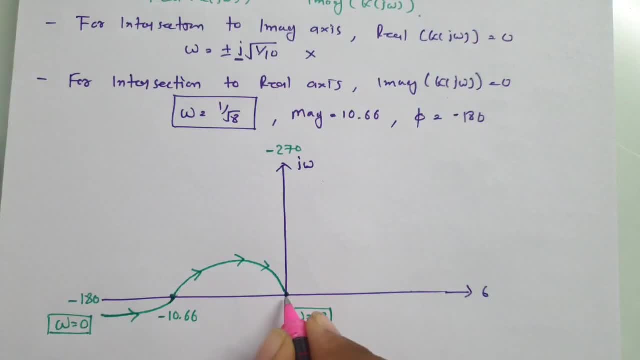 to have in anticlockwise direction. So I will have to make 1.5 circle in anticlockwise direction. So you see, this is one circle and this is another circle in anticlockwise direction. It is bit difficult to show with 0 radius. 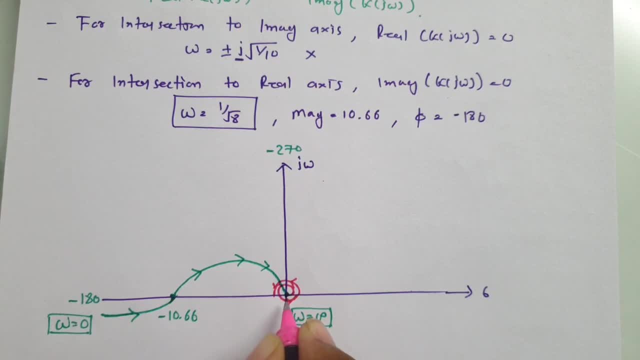 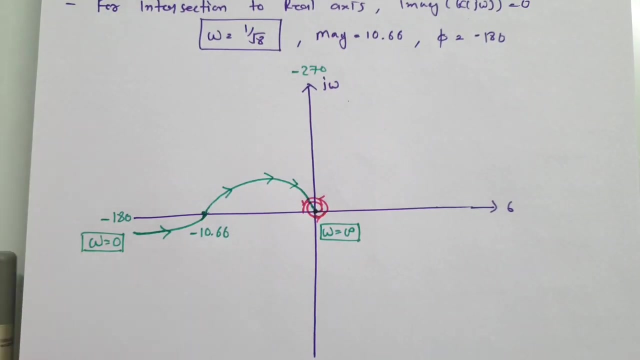 But 1.5 circle. that is happening with anticlockwise direction, with origin right Now, if you see third step, So that is to have inverse polar plot. So let me show you how to have inverse polar plot, So it will be exactly opposite. replica of this. 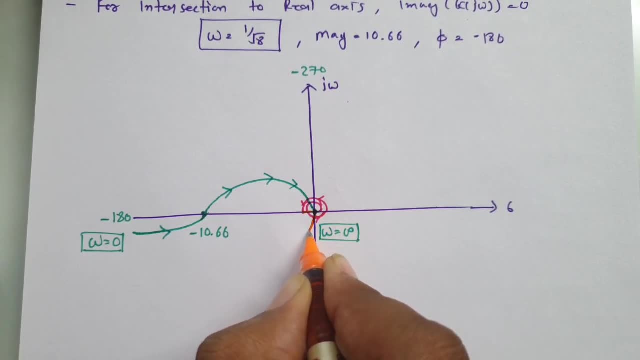 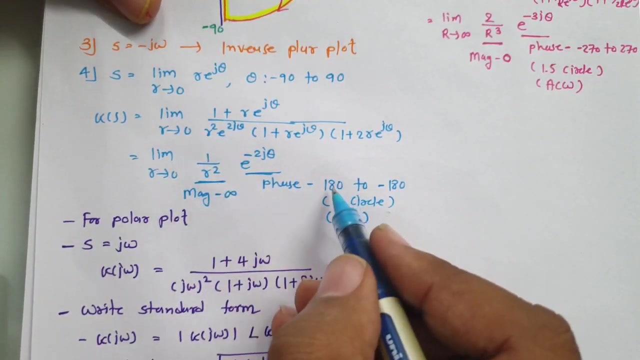 So you see, that is happening like this, This, This, This, This, This. That is happening like this. So this is exactly opposite replica And if you observe, if you observe final point, so that is having magnitude, infinite radius and it is starting from 180. 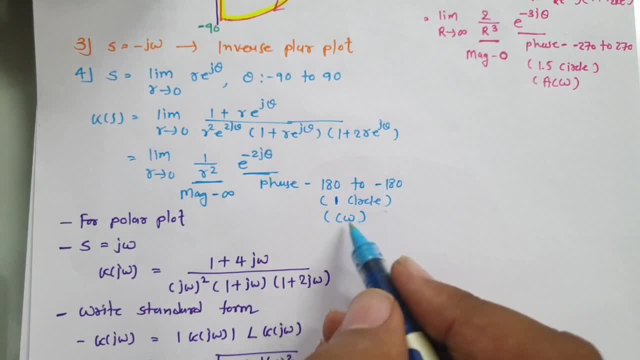 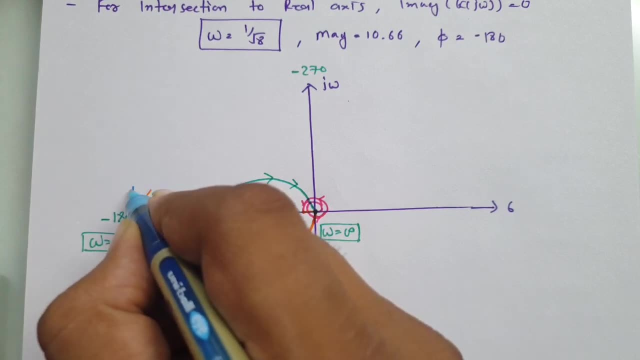 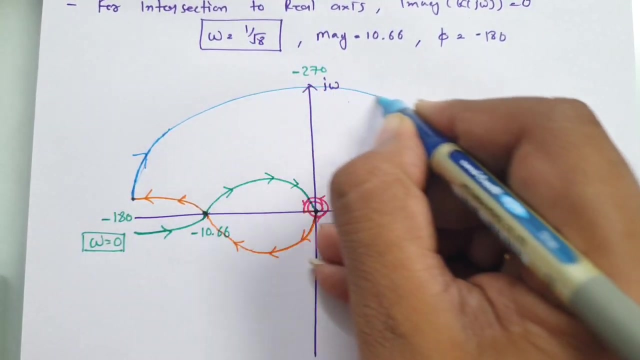 to minus 180, right, In clockwise direction. So you see, now it is happening up to this, Now it will be having 180 to 2 minus 180.. Right, So it is happening. Okay, in clockwise direction. so this is how it is happening from here and it will be having. 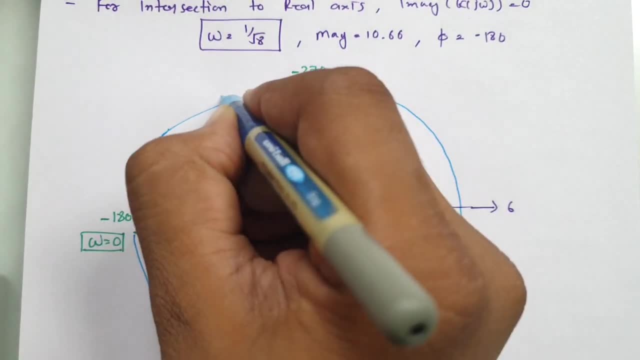 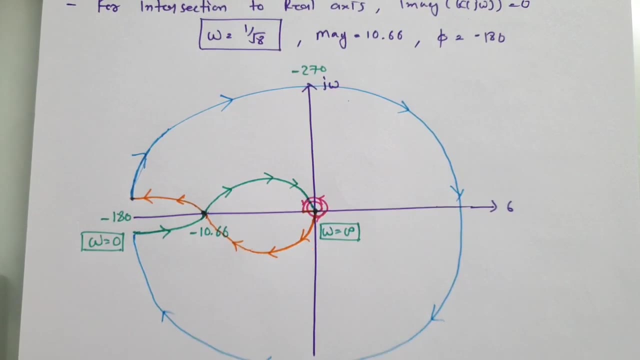 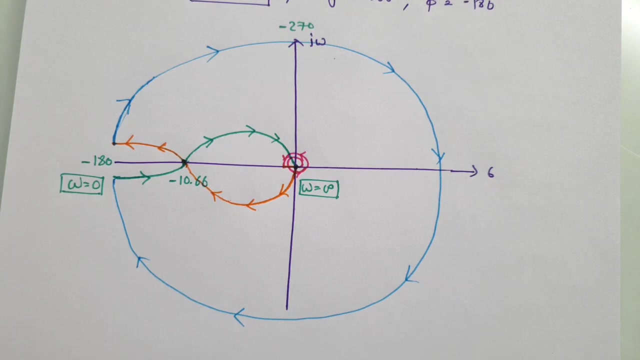 infinite radius circle and it should be there in clockwise direction, and there is a one circle it will enclose over here, right? so that is how complete nyquist plot that is there with us by four sections, which i have explained. now there is one more question, that is a stability. 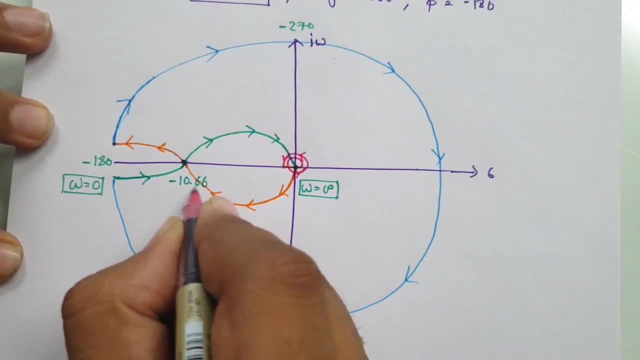 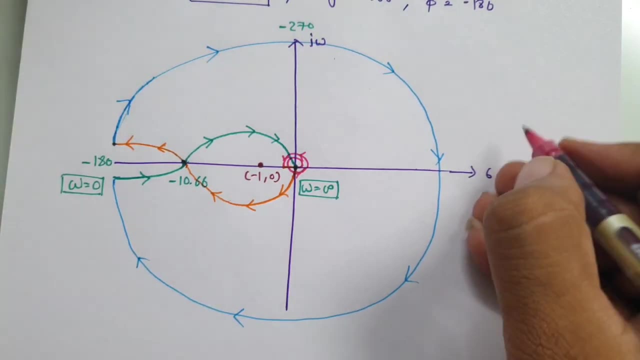 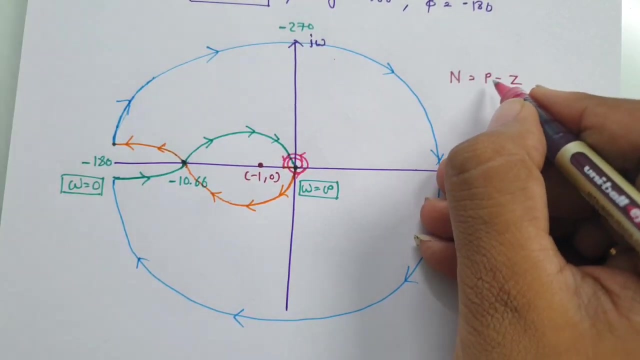 right now. you see this is minus 10 comma, minus 10.66. so critical point, let us say it is minus 1 comma 0 somewhere over here. so stability that we identify as per n is equals to p minus z, where n is encirclement, p is number of poles for open loop transfer function and z is number of 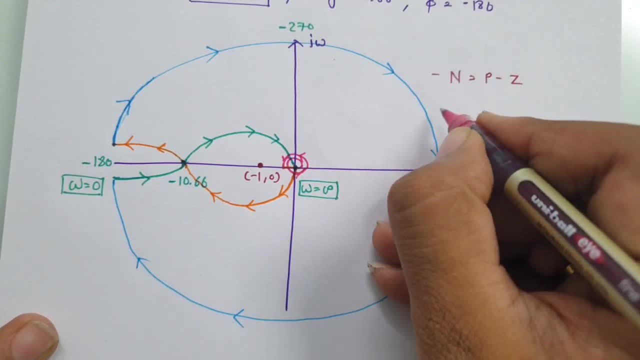 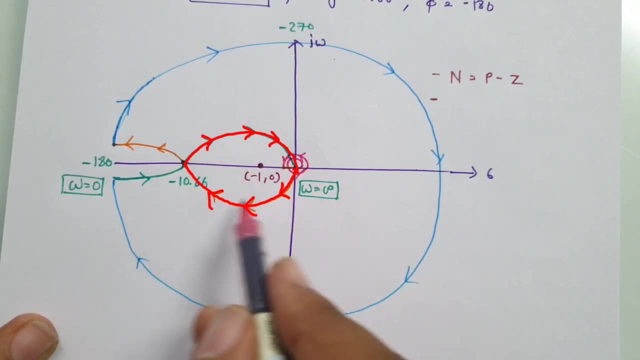 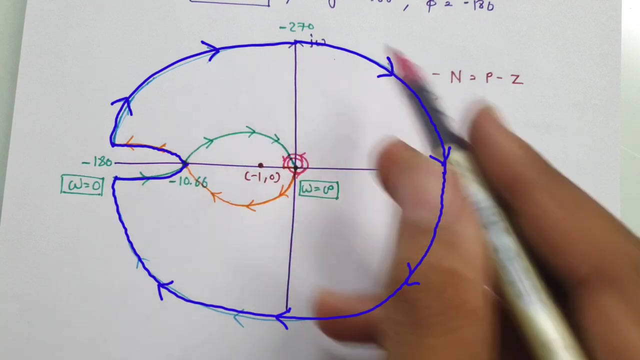 poles for closed loop transfer function. now, what is n over here? so n, you see encirclement of this minus 1 comma, 0 point. so this is one encirclement in clockwise direction and this is second encirclement in clockwise direction. right, so two encirclement in clockwise direction is happening.